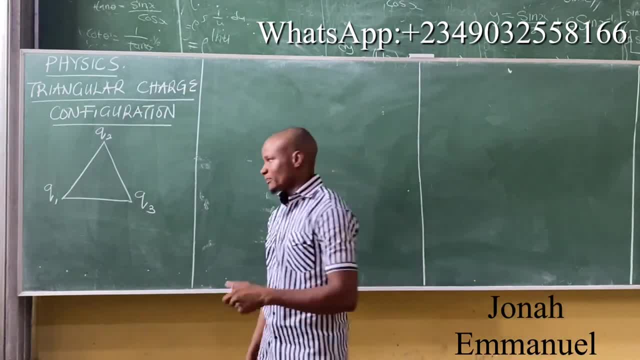 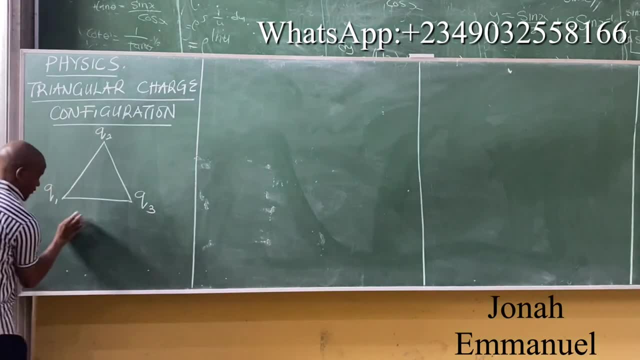 Let's do an example. please Take that book Example: Example: Three charges. Example: Three charges, Three charges: 14 microcoulium, 35 microcoulium and minus 27 microcoulium Three charges. 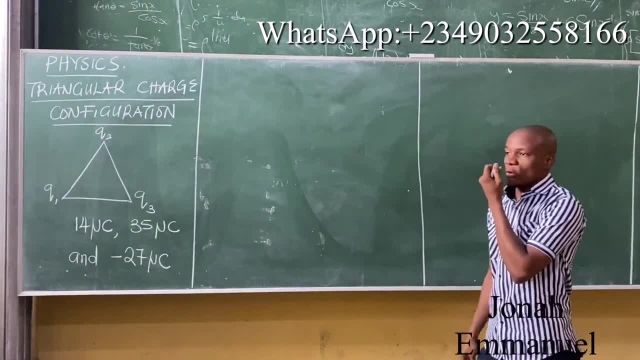 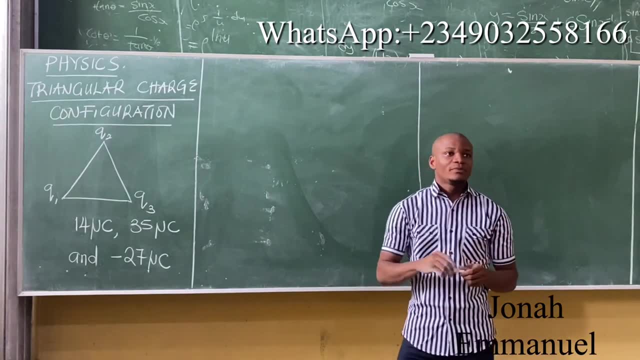 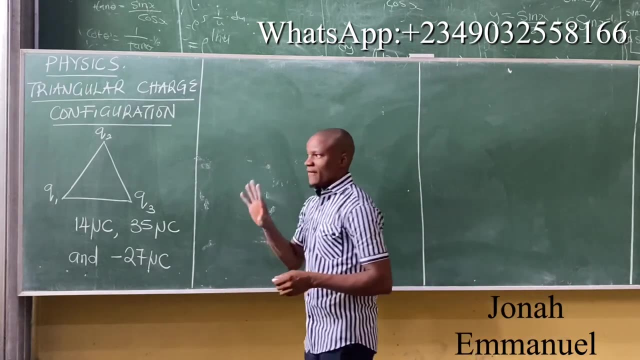 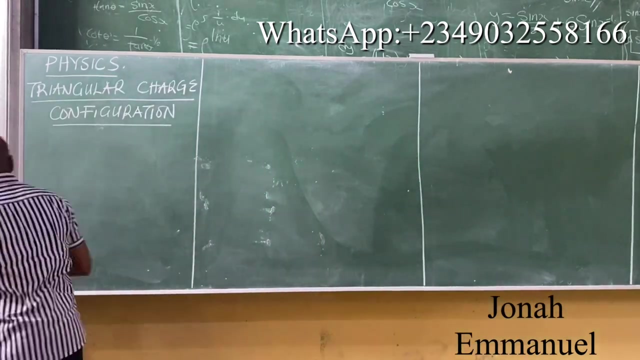 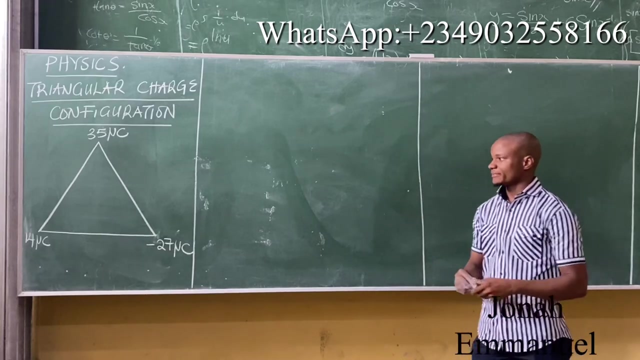 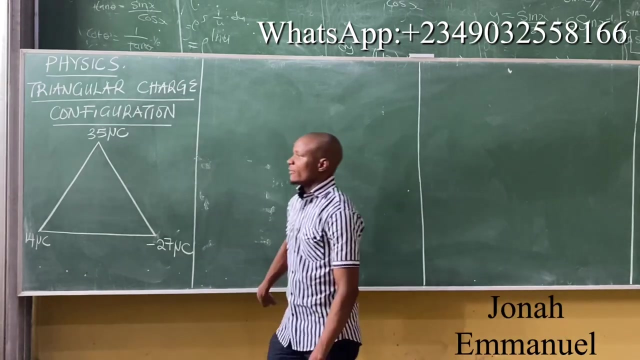 14 microcoulium, 35 microcoulium and 27 microcoulium are arranged along the vertices of a triangle. Are arranged along the vertices of a triangle as shown below. As shown below This: Find the resultant force on the 14 microcoulium charge. Find the resultant force on the 14. 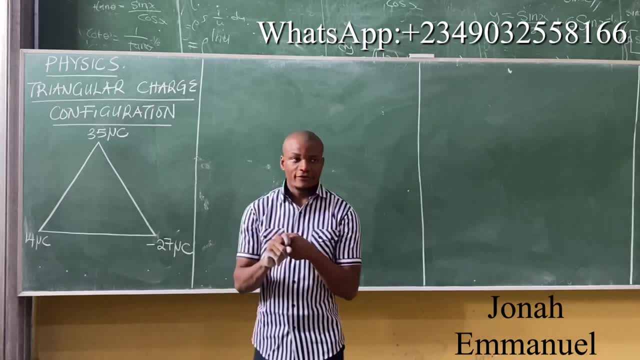 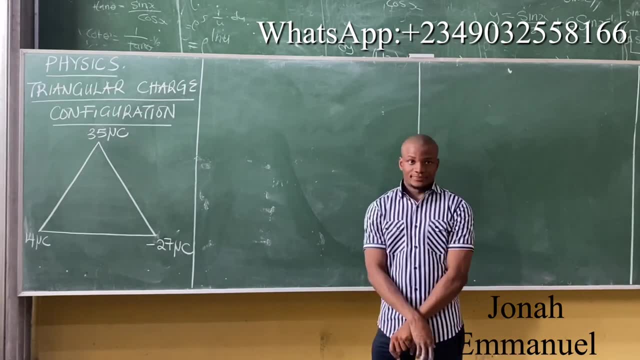 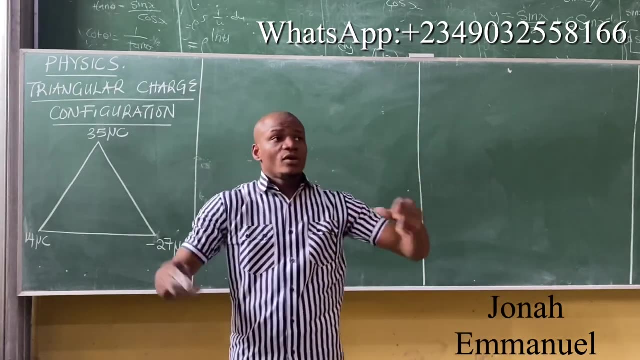 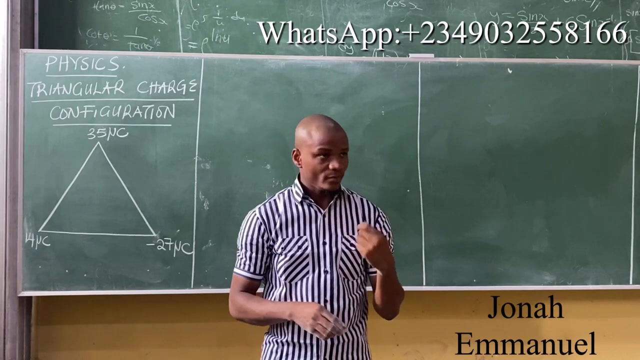 microcoulium charge. On the 14 microcoulium charge: Alright, Solution, please, Solution please. So I said your first task is always to get out Q1,, Q2, Q3.. In some question you'll think: 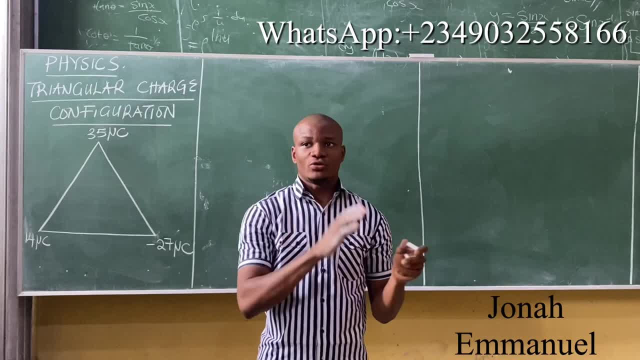 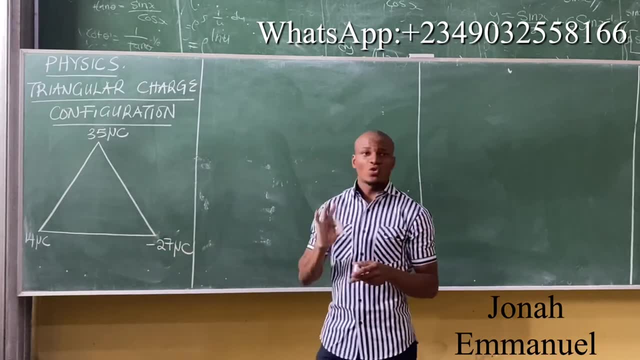 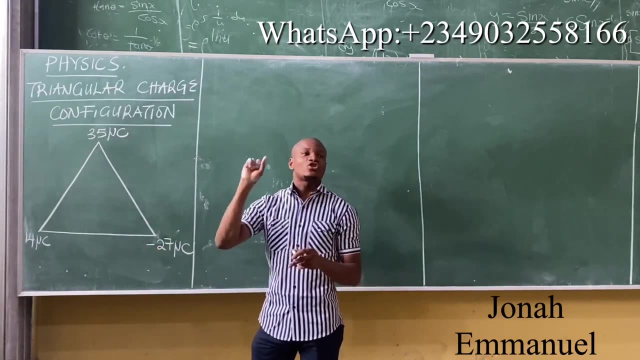 that Q1 is equal to something, Q2 is equal to something, Q3 is equal to something. In this question, we're not given Q1,, Q2, and Q3.. We're just given just these three charges there. So your first task is to assign Q1,, Q2, and Q3 to any one of these three charges. 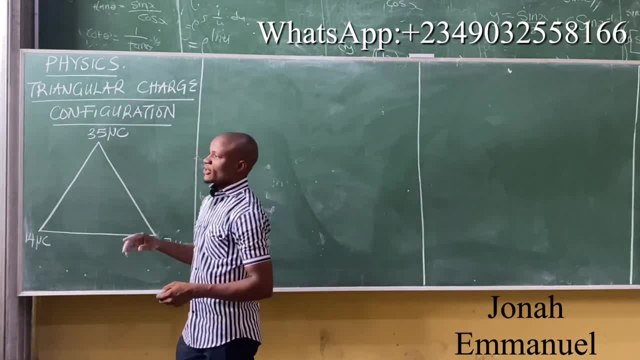 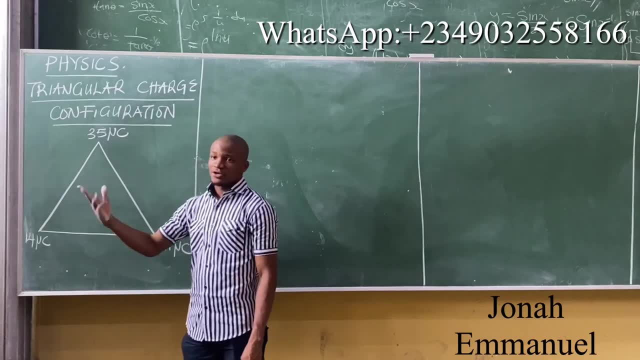 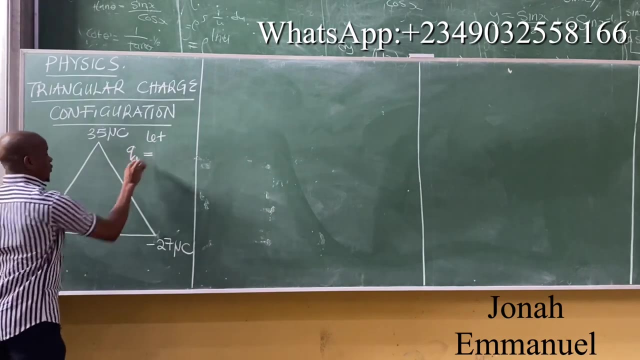 Any one you choose to. Now here's the argument, The ask to find the resultant force on this one here, And I would advise that always call this one what there, Q1.. That's all. So case one, Let's. let's Q1 be equal to this 14 microcoulium, Q2 be equal to this minus 27 microcoulium. 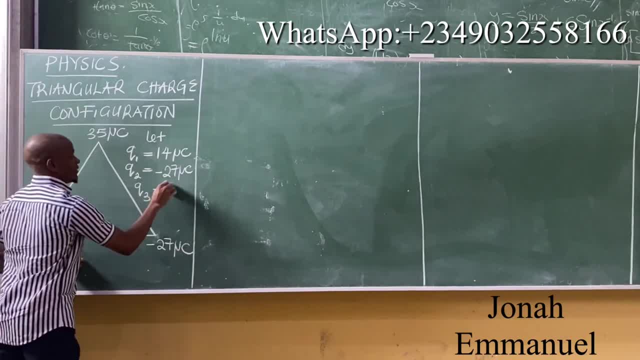 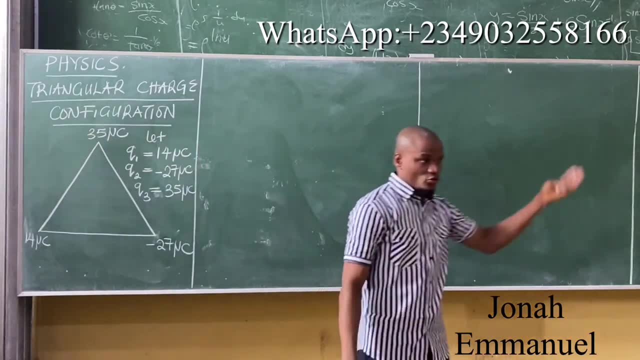 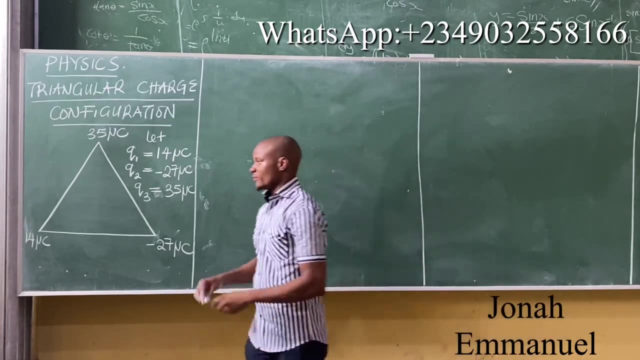 And then Q3.. B equal to this one here, 35 microcoulium. Alright, So assign this one. Let Q1 be this, Q2 be that and Q3 be 35 microcoulium. The ask to find the resultant force on this one. 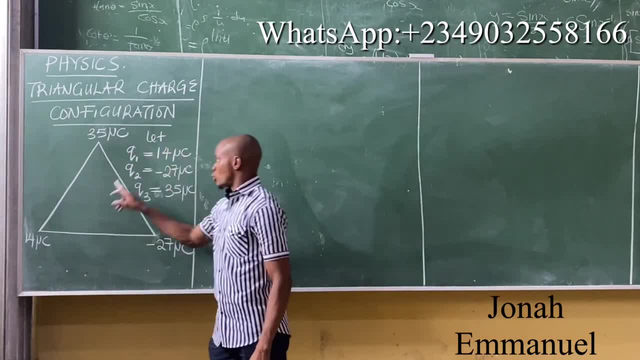 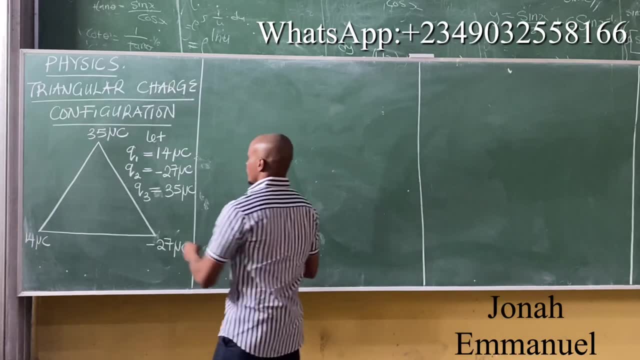 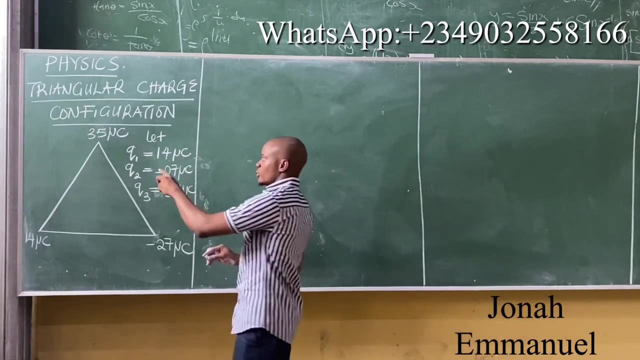 here. Alright, Of course we call this Q1. So take that one. The resultant force on Q1, which is 14. Set on 14.. So this is Q1. The resultant force on Q1 is given by: So we set F1 resultant. 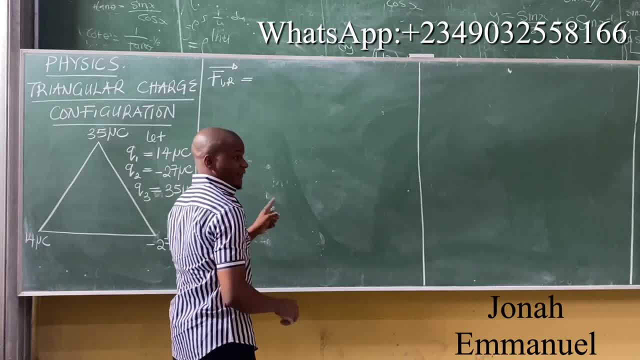 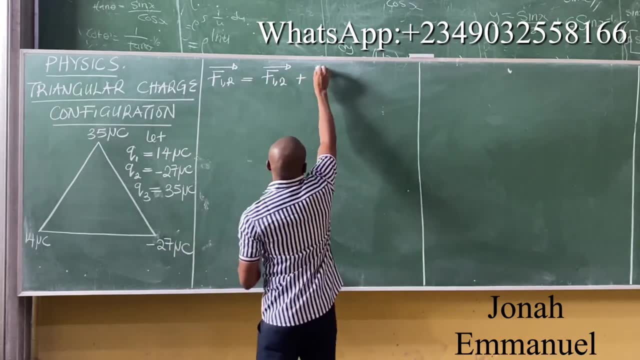 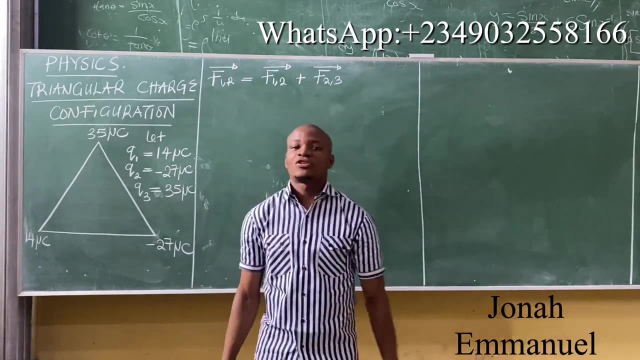 is equal to F1- 2 plus F2, 3.. So it becomes F1- 2.. F1- 2 plus F2- 3.. F2- 3.. Please, if you missed our last class, alright, the video is already online, but I'm not releasing it. 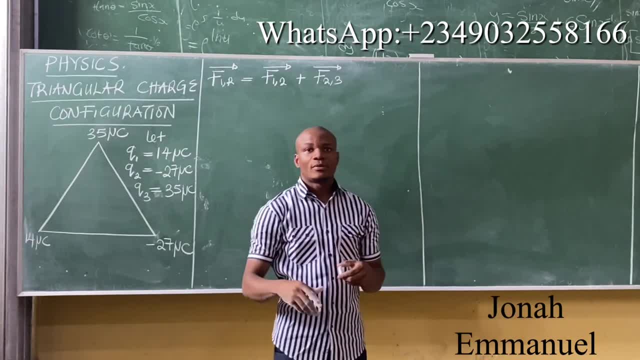 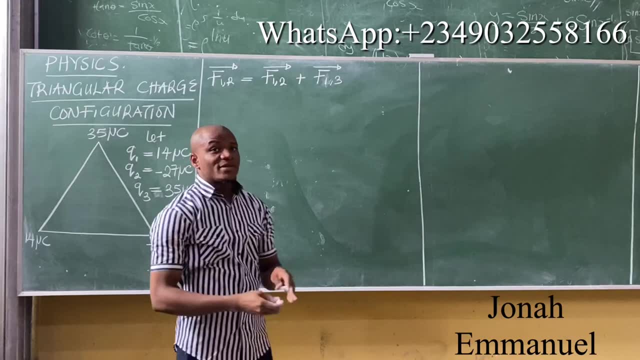 here on how we derive all this stuff. 1, 2, and F1, 3, please. F1, yes. So if you missed our last class, because I'll upload the video, it's already online, I'll just release it, perhaps. 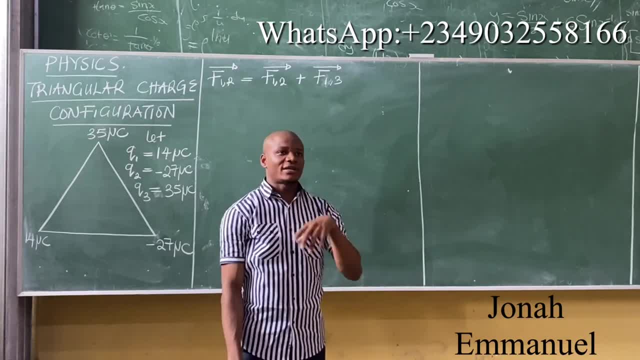 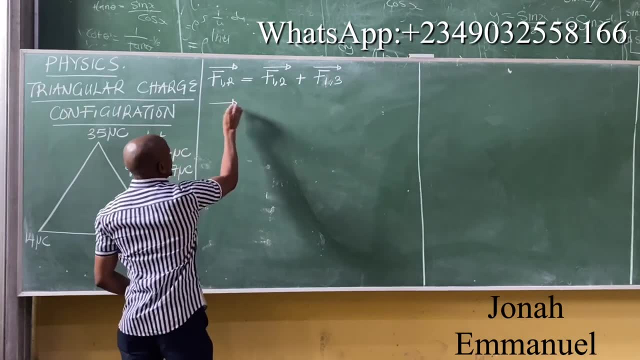 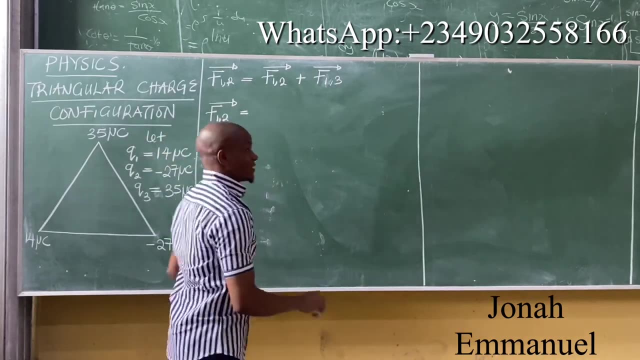 today, this evening or tomorrow. So please check out our last class and see how it works this stuff. Alright, let's get F1, 2.. So F1, 2 is equal to. from Columns law we said F1, 2 is K. 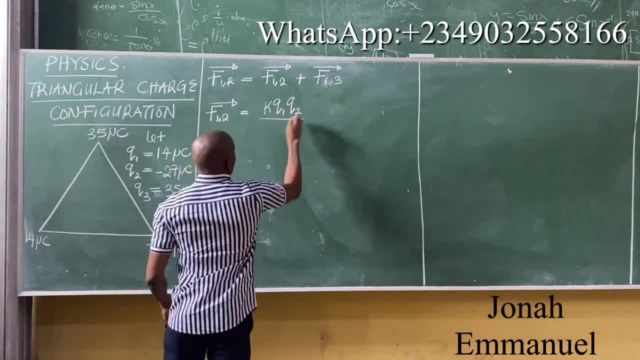 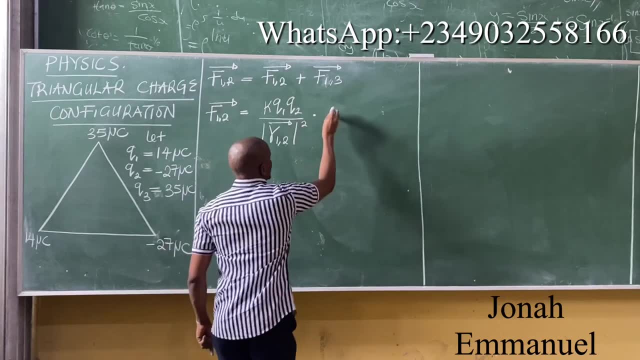 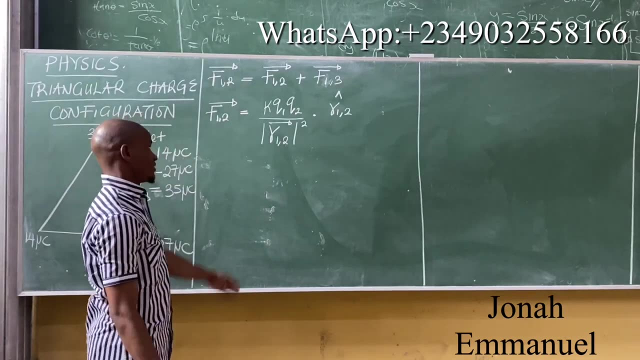 Q1, Q2 all over R1, 2. this all squared dot the unit vector of R1, 2. So this is F1, 2. Here's your formula from Columns law in vector form. That's what Next up we said. 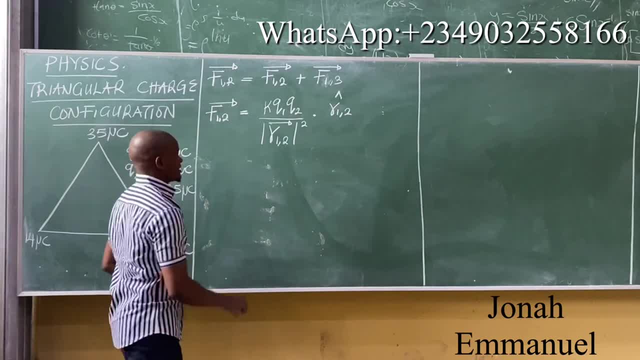 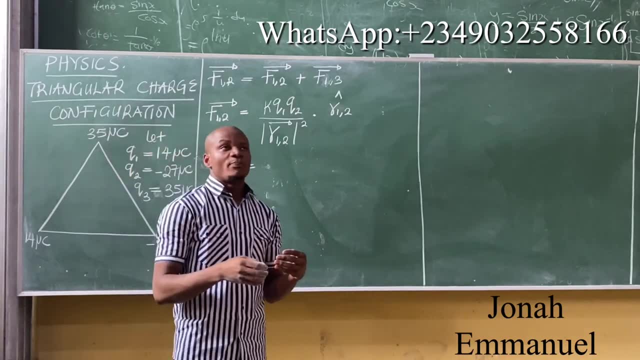 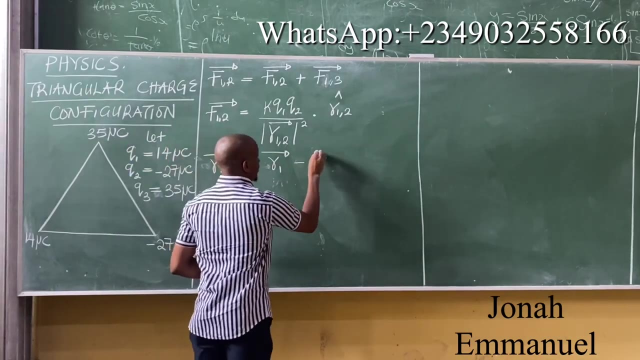 you start by considering this first. So let's go with R1, 2.. R1, 2, we said, is the difference between the position of charge 1 and charge 2.. So R1 becomes R1 minus R2.. So having R1, 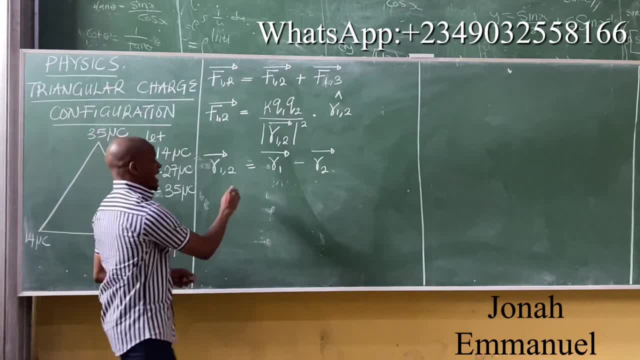 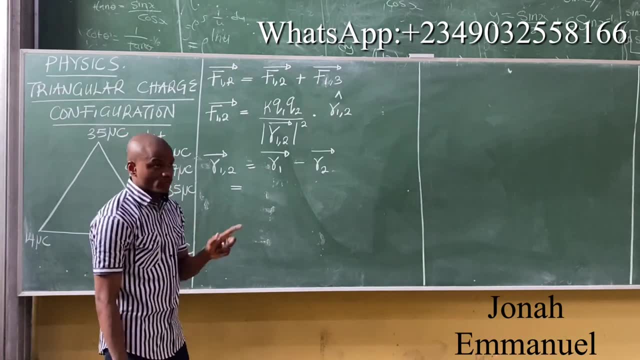 minus R2.. So I have this. We said R1, the first one here is always considered as the origin, So it becomes 0. So R1, here it becomes 0. Minus Let's get to R2.. 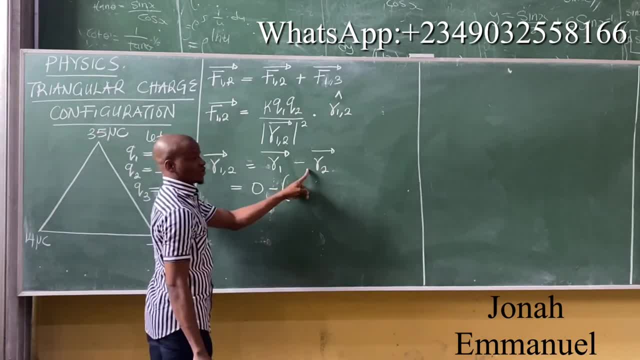 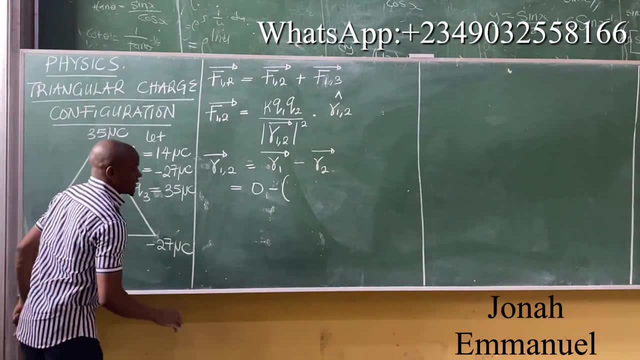 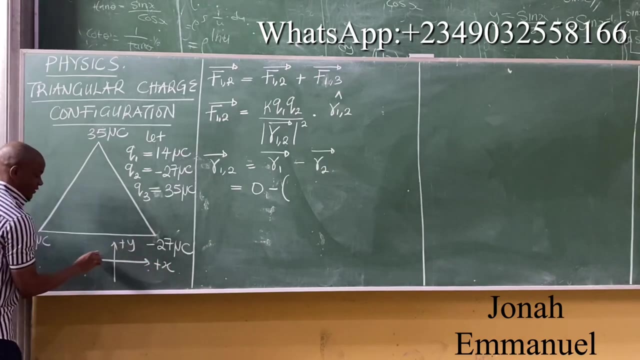 So we said for this one here, when it comes to getting this position, I said your first task is to compare this to the Cartesian coordinate. In my Cartesian coordinate system I have this: This is positive X. This is positive Y. This is negative X. 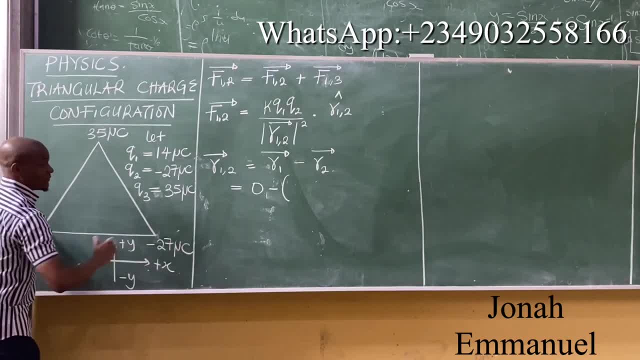 Here is negative Y And I said moving to the right. if I'm going to the right, that is positive, So it becomes plus, If I'm going to the left, that's negative. If I look at R1, which is this: 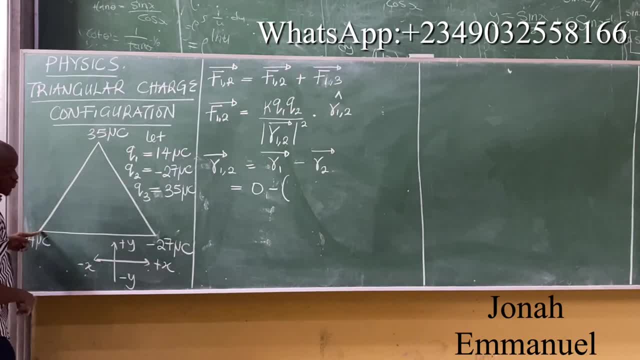 the position of Q1, which is this minus R2.. R2 is here and it's at my right For me to move from here to here, I have to move to the right And we said: if you're moving right. 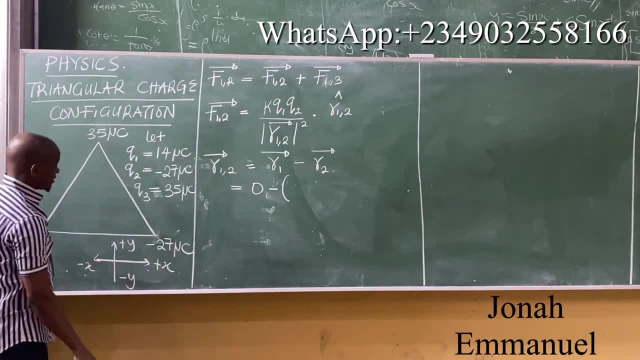 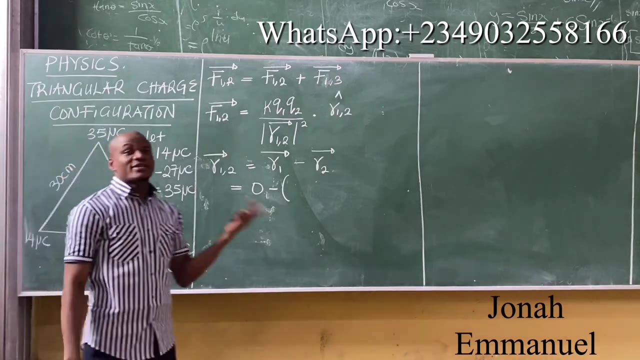 it becomes what there Positive, So it becomes plus. Will we give you distance? No, Sorry, please. Our distance means Let's take care. Let's take care of 30 cm, Let's take care of 30 cm. 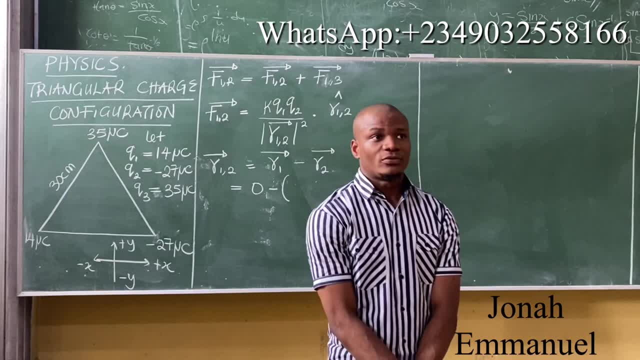 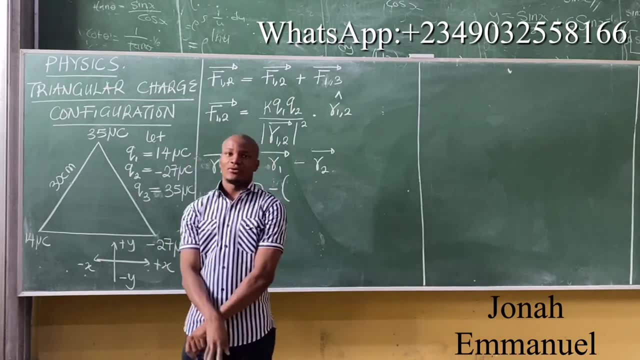 and assume the triangle to be an equilateral triangle. We're taking care of 30 cm and we're assuming the triangle to be an equilateral triangle. Of course, for an equilateral triangle, you only need to give it one side. 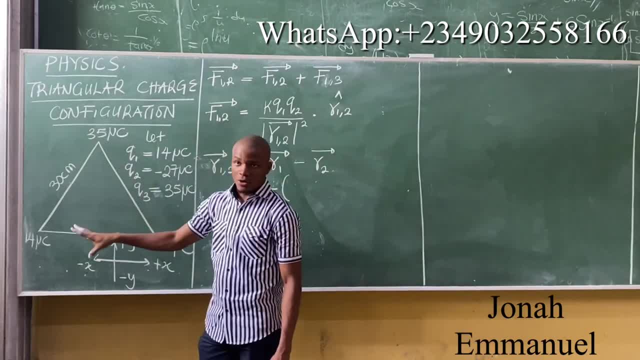 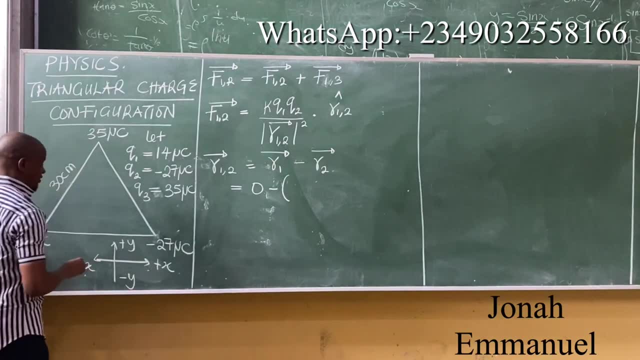 Because if it's equilateral, that means all the sides are equal. If here is 30, here becomes 30.. Here becomes 30. Of course, from what cm to meters It becomes what? there? 0.03 meters. 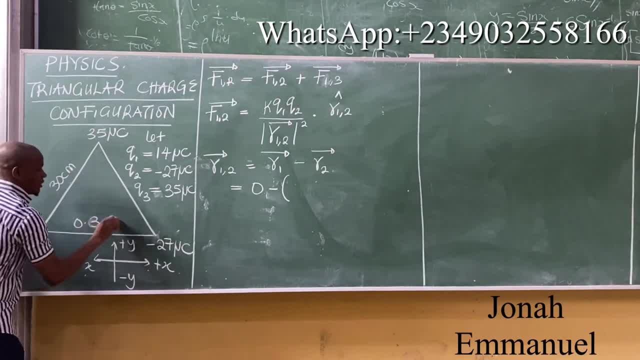 0.3 meters Divide by 100, gives you 0.3.. Alright, So I'm here minus R2.. For R2, I'm moving to the right. So it becomes positive. So it now becomes plus. 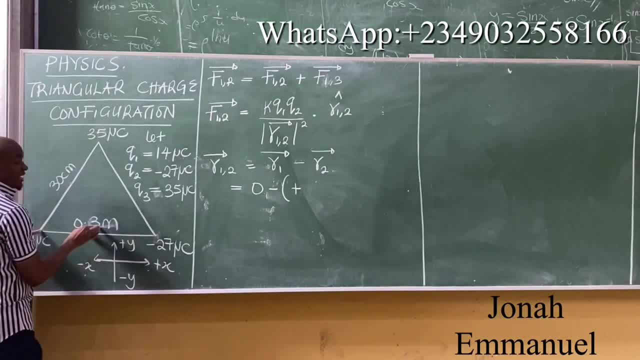 From here I'm moving this distance. Distance here is 0.3.. So it becomes 0.3.. Next up it's in the X direction. We said: for X direction, call it I. For Y, call it J. 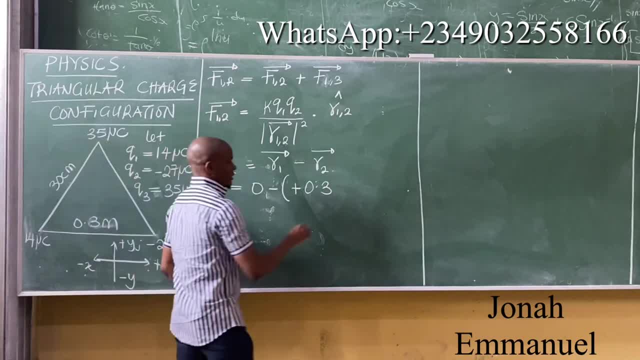 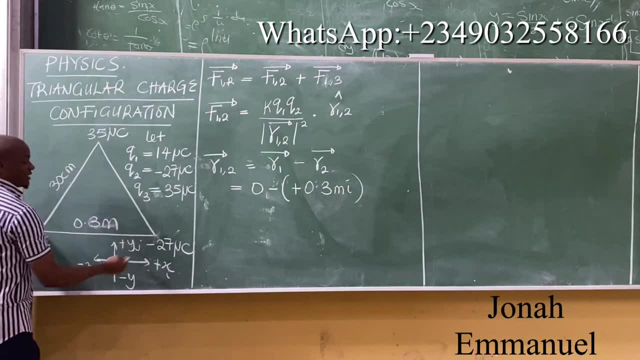 So, since I'm moving in the X direction, it becomes I meters. Ah, so I have this. So it becomes 0.3 meters in the I direction, That's X direction. So I have this. Expand the brackets. I'm having minus, so this becomes minus. 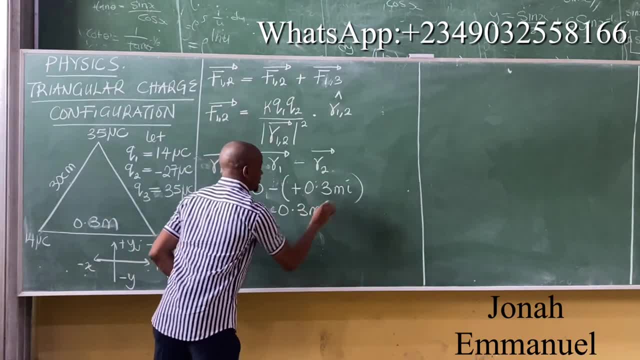 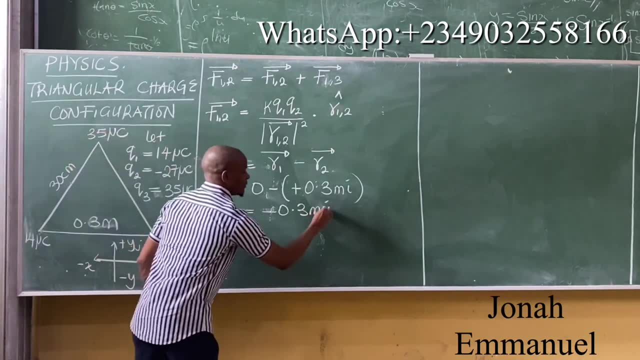 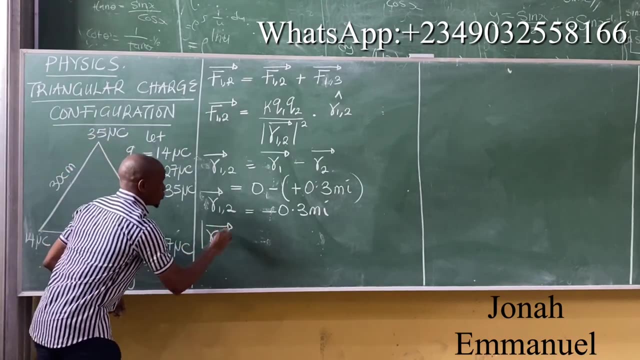 I'm having minus 0.3 meters I. This is R1, 2.. So we said after this, of course I, We said after this: your next task is to get the magnitude. We said the magnitude of R1, 2. 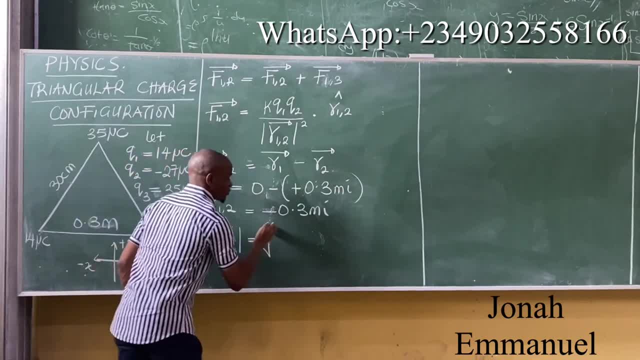 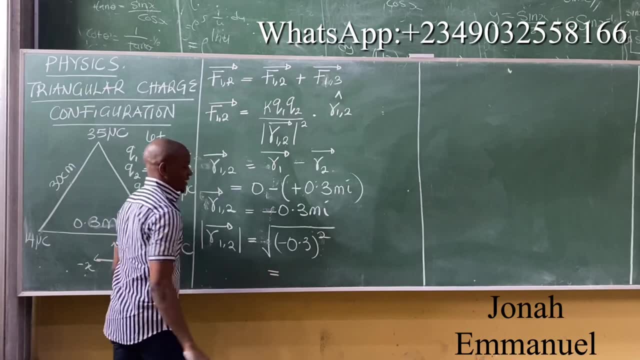 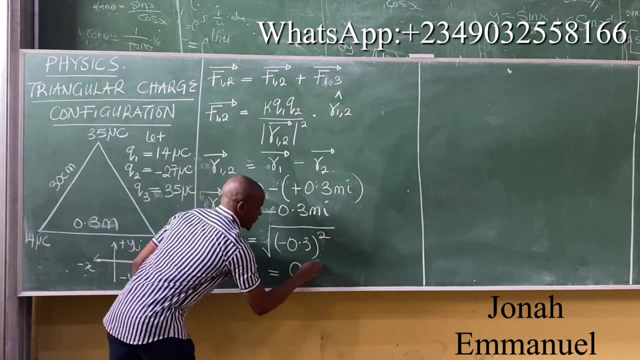 is equal to take the square root of this term minus 0.3 squared, And from our last task we said this square will cancel the minus And of course, gives you the same term there: 0.3 meters. 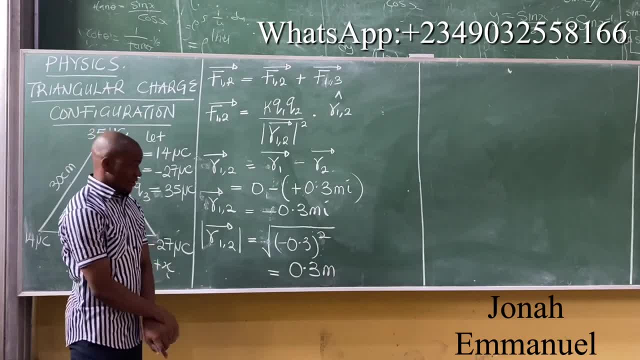 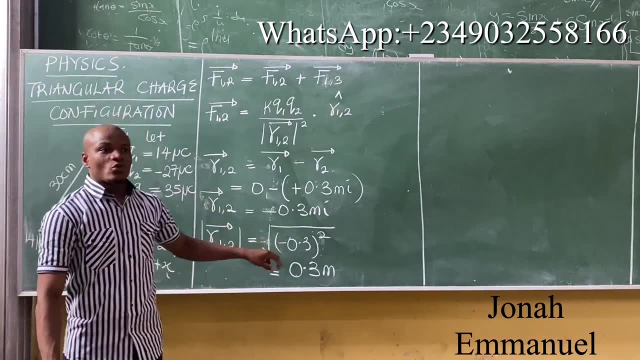 So I have this as my answer: If you square this, you have this case here. If you heard the last slash, no, thank you. Who doesn't know why I'm having 0.3 here? Who doesn't know why? 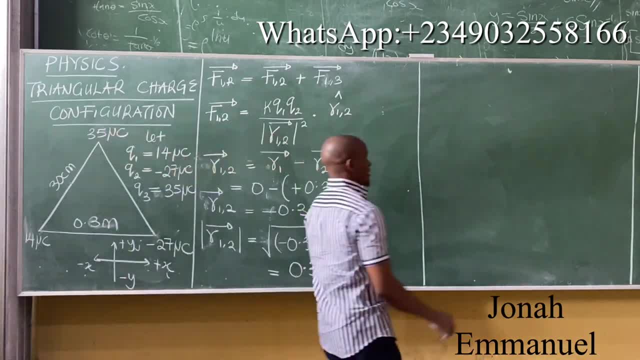 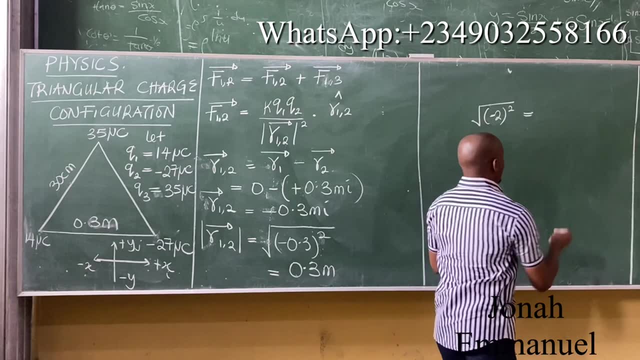 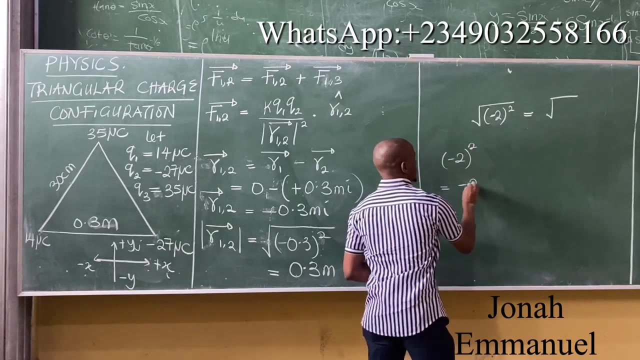 You don't know why. Two results: Square root of. look at this. Let's say minus 2 squared, for instance. Work this out step by step. This gives you the square root of minus 2 R squared. minus 2 R squared is equal to minus 2 times minus 2.. 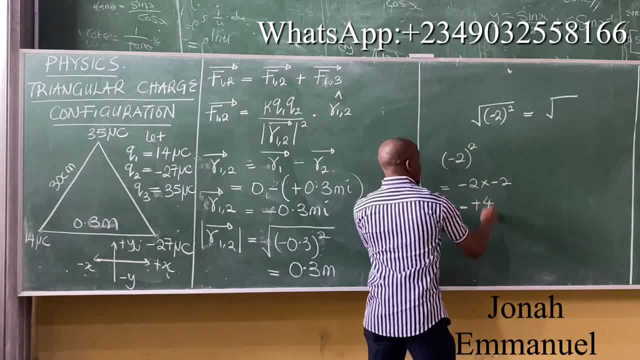 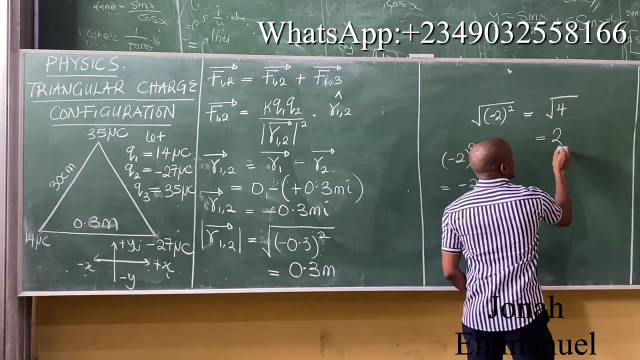 And that's equal to minus times minus is plus 2 times 2 is 4.. So minus 2 R squared gives you 4, is equal to square root of 4 is 2.. So observe that this cancels this. 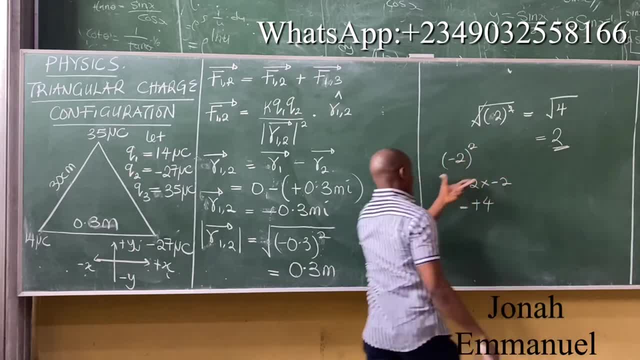 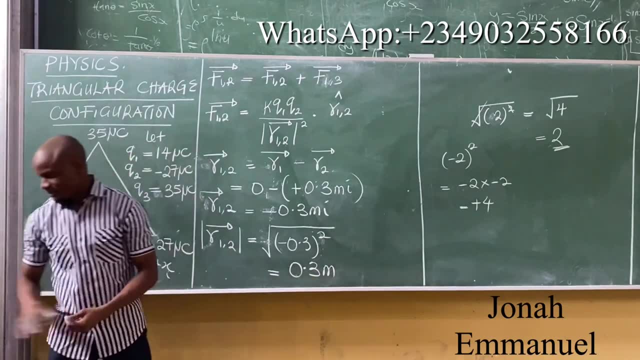 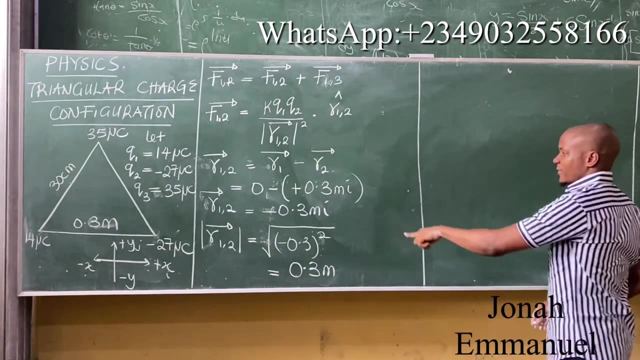 and the minus goes up. I'm having 2.. This same idea is used here, So this cancels this, and the minus also goes up. So I'm having this. So that's the concept here, All right. Next up, get unit vector. 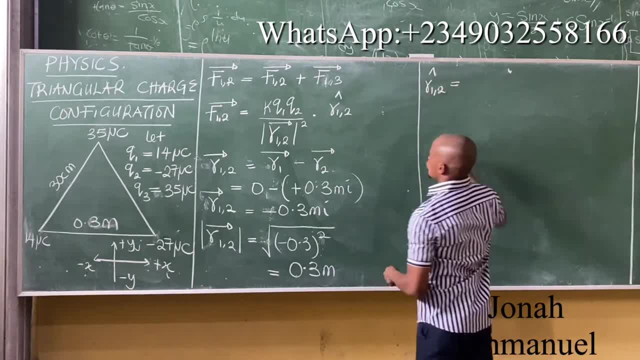 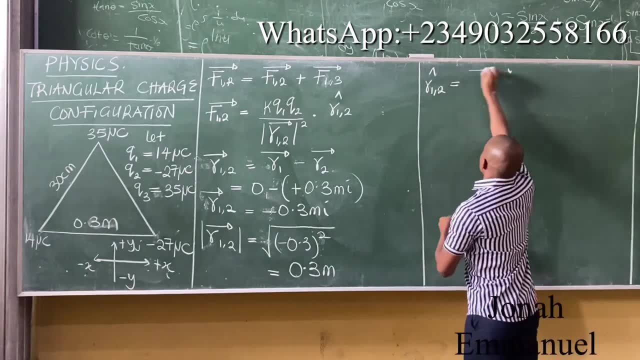 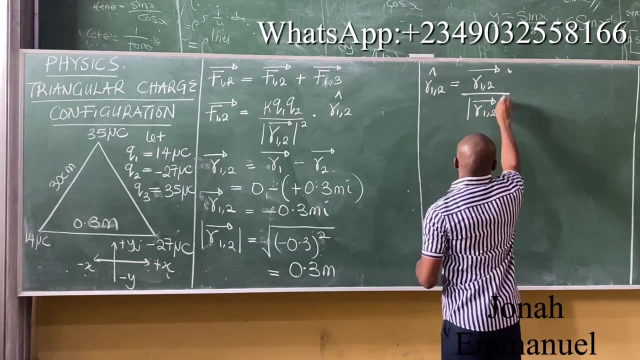 So unit vector of R12. We said unit vector is the ratio of the position vector all over the magnitude. So it becomes position vector R12 all over the magnitude of R12. And that's equal to position vector of R12 is this: 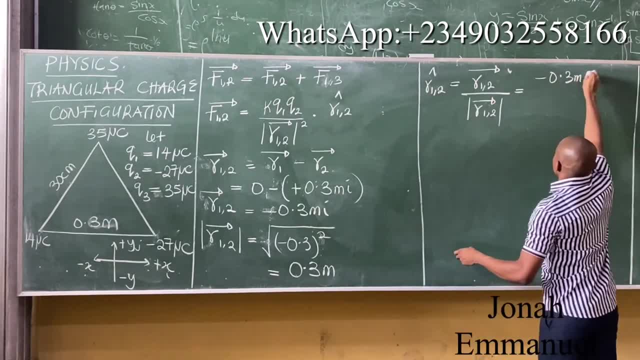 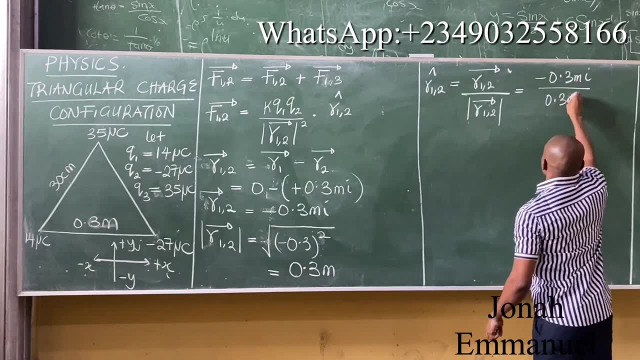 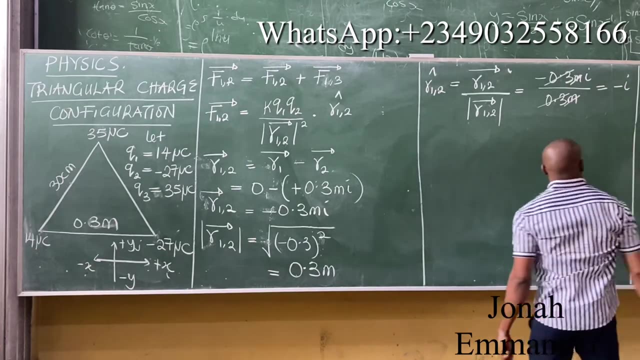 That gives you minus 0.3 meters high all over. The magnitude is what we got here And that gives you 0.3 meters From here. this cancels this. Meters cancels meters is equal to minus R, So we have this. 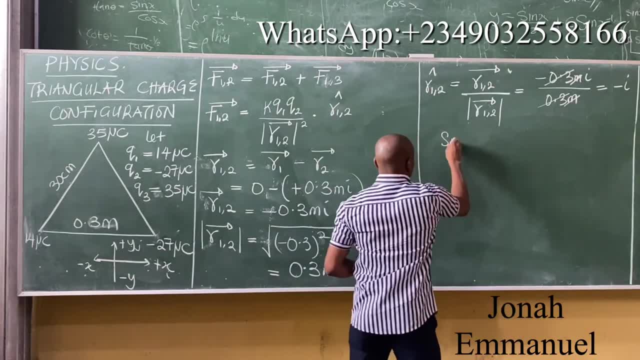 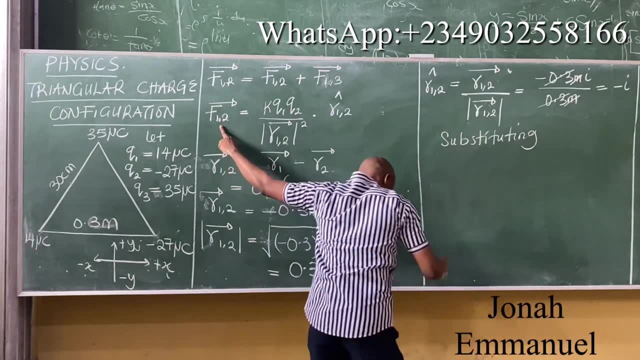 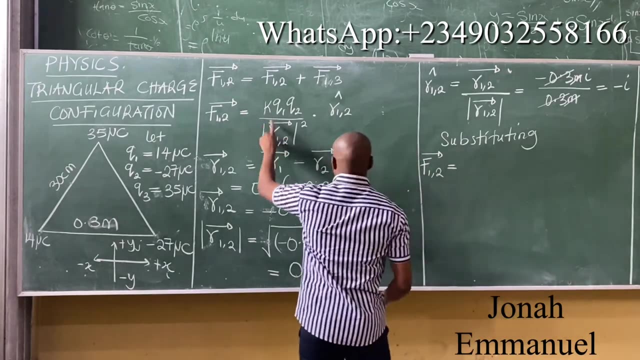 Finally, substituting, Substituting, Substituting, Substituting, Substituting: I have that F12, this I have that. F12 is equal to k. k is constant, That's 9 times 10 to the power 9.. 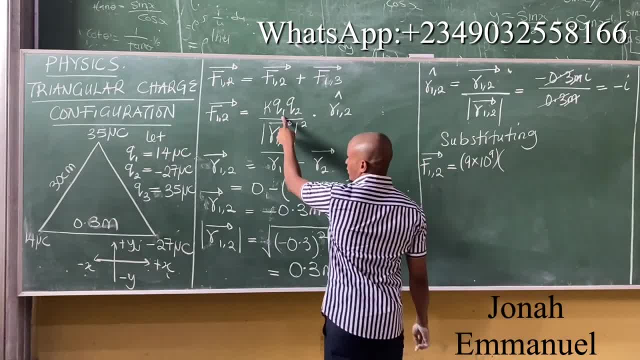 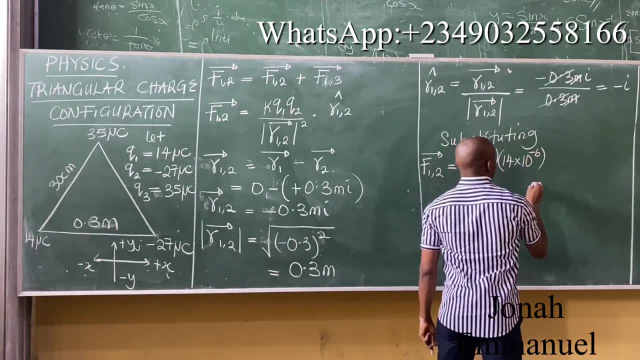 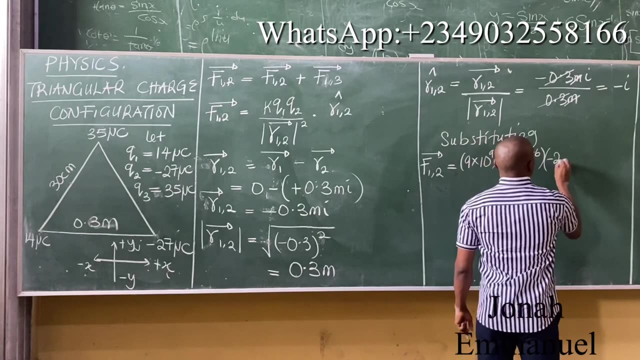 That's k. Into q1.. q1 is 14 in micro. That becomes 14 times 10 to the power minus 6.. Into q2.. q2. Q2,, which is this minus 27,. minus 27 micro, that becomes times 10 to the power minus 6.. 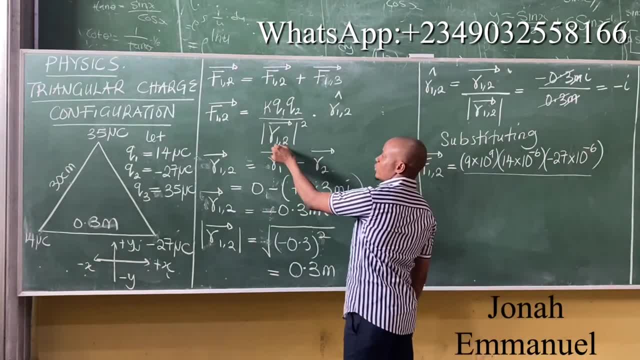 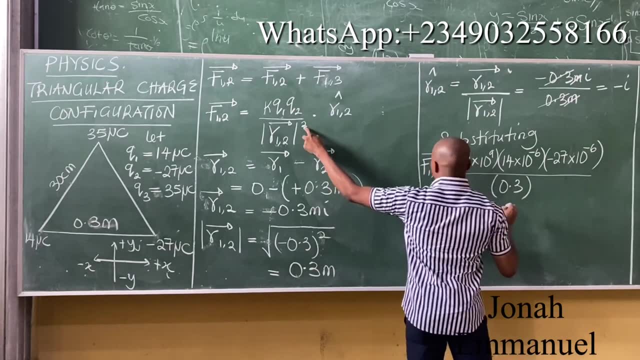 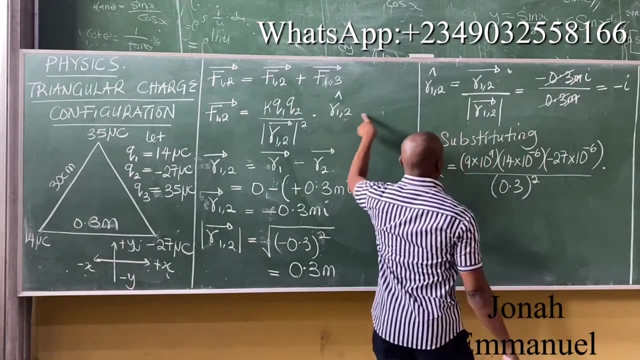 All over. next one says magnitude of R12. This value is what we have here as 0.3.. So it becomes 0.3 percent squared. So I'm squaring this dot R12, the units vector of R12, which is this as minus R. 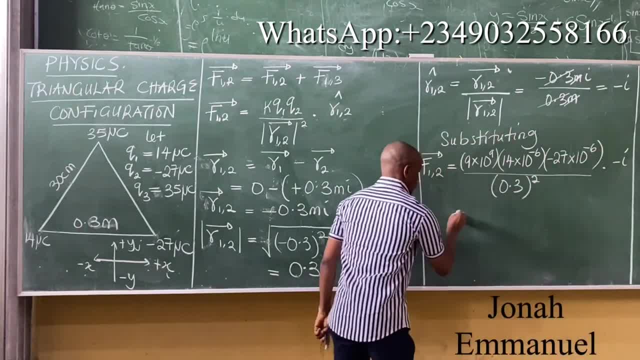 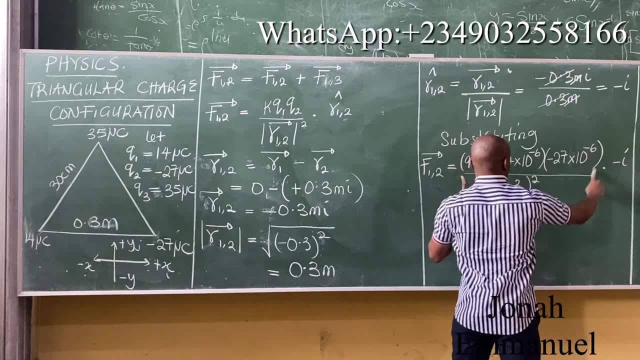 So I have minus R, Alright, so F12 is equal to give me all of, in fact, give me everything here. what do you have? Give me everything here. what do you have? Watch everything here. what do you have? 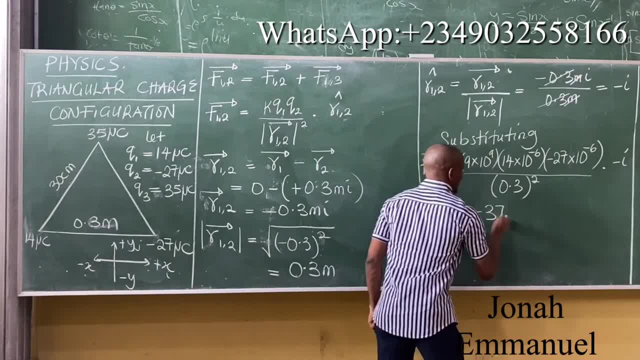 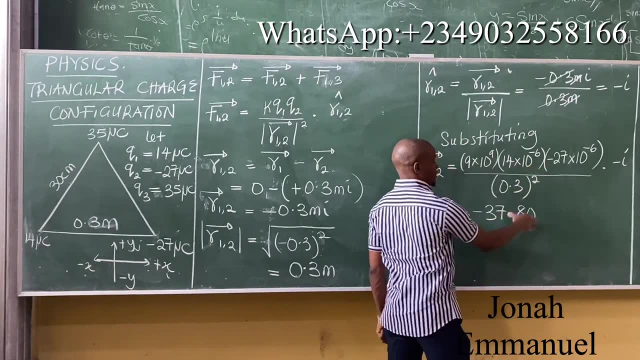 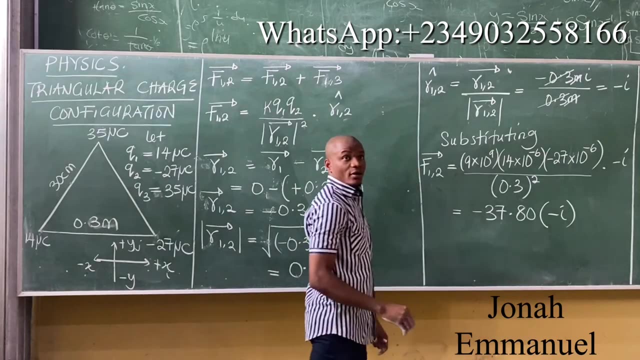 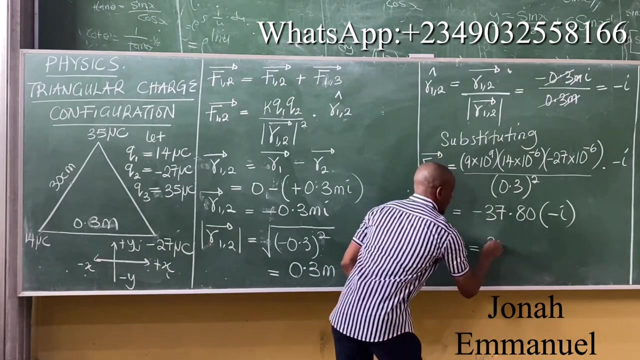 So this gives you minus 37 points. In 2dp it's 0.. Alright, so this one gives you this into. I'm having here minus R, Alright, Hope it's correct. Alright, So that's now equal to minus minus dc plus. so this now gives you 37.80, it's plus. 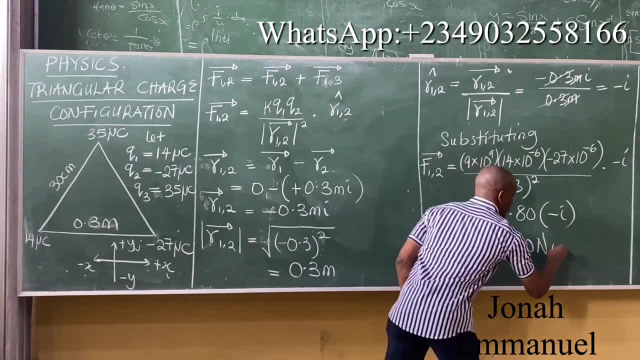 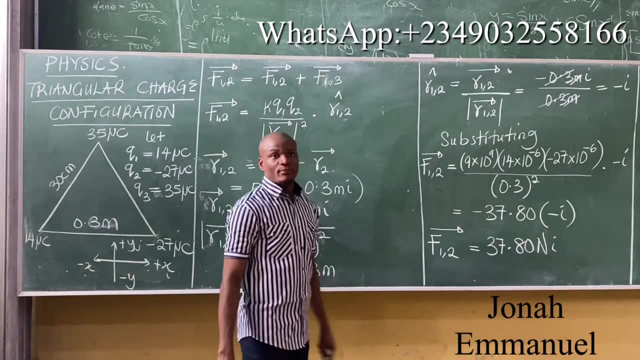 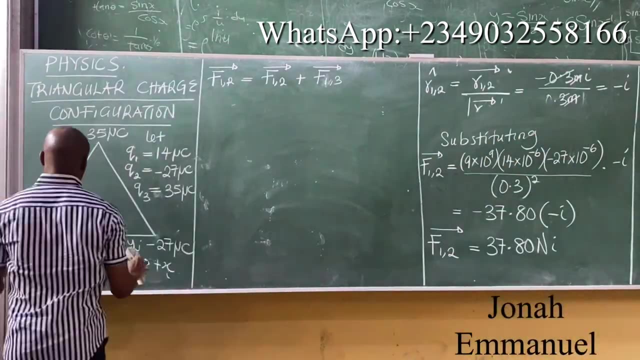 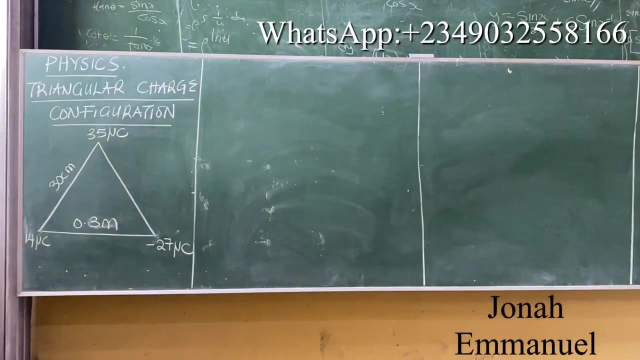 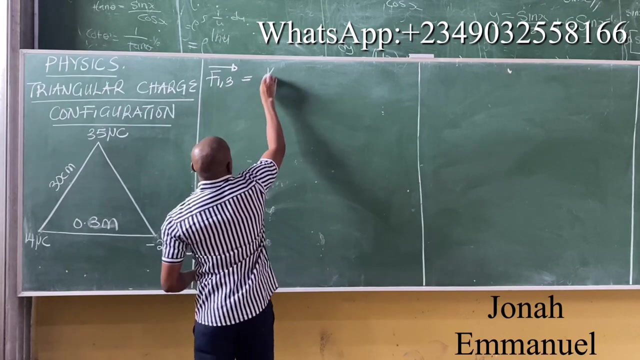 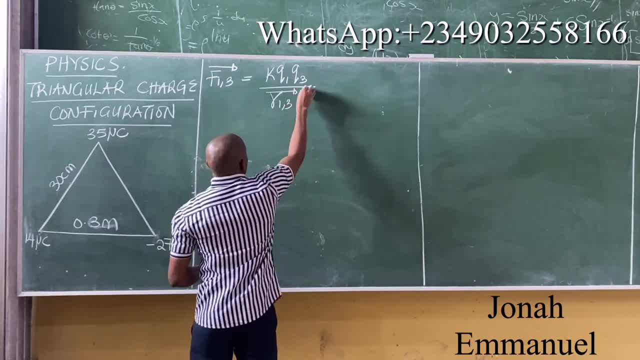 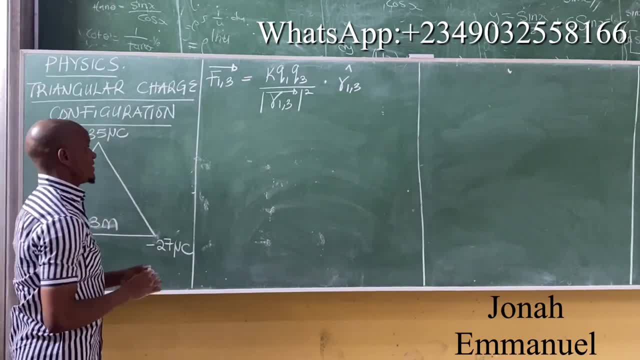 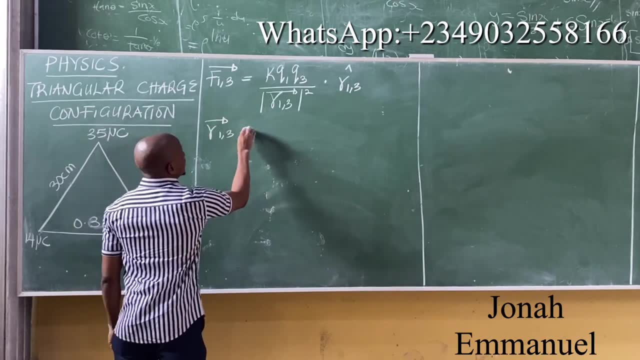 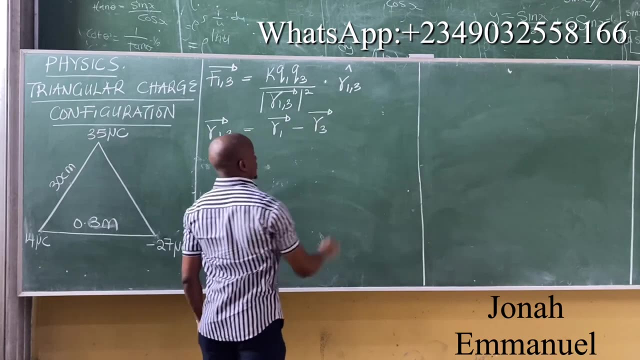 So I have this. So we said: first is first. Your first task is to get this value. Let's get R13.. R13. So R13 is equal to R1 minus R3.. So I'm having this one there. So we said: this one always be your. 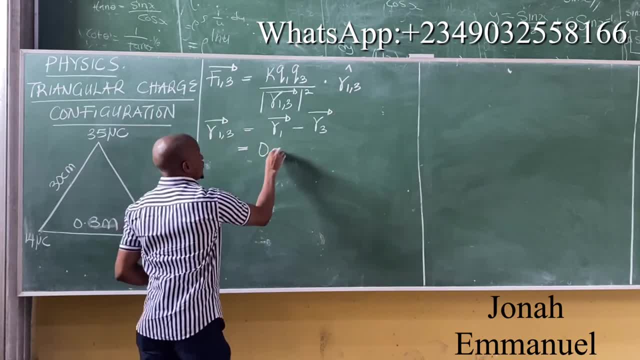 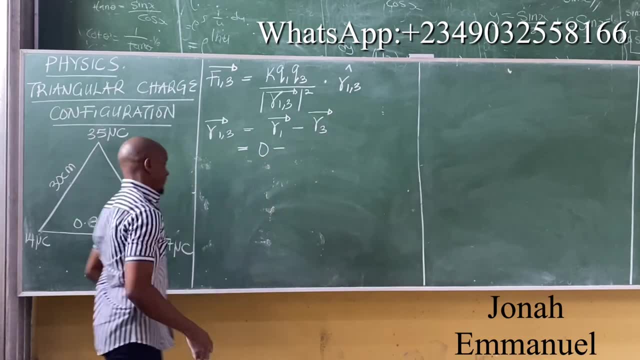 So we said this one: always be your origin, which is 0.. It becomes 0 minus. next up is to get the position vector of charge 3.. That's R3.. Now look at this. Look at this. This is R1.. 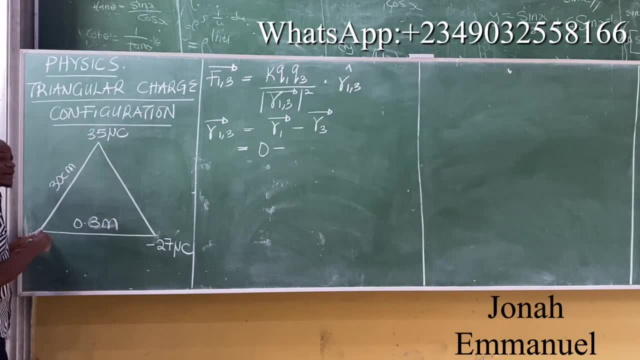 We said: distance from R1 to R2 is this one? yeah, 0 point. We are giving 30 cm. Combating to meters, we have 0.3 meters Of course, So here also becomes 0.3 in meters. 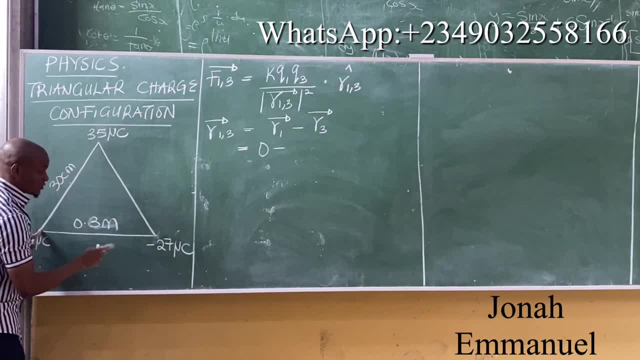 Here also becomes 0.3 in meters. So this is R1.. This is R2.. This is R3.. This is R2.. This is R3.. This is R4.. This is R5.. This is R6.. 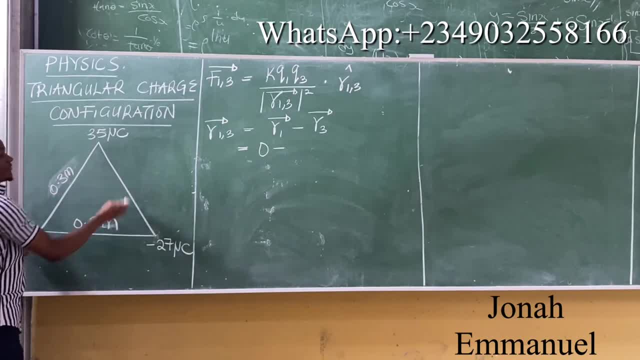 This is R7.. This is R8.. This is R9.. This is R10.. So we have 0.3 meters. So distance from charge 1, which is this, to charge 2, is 0.3.. 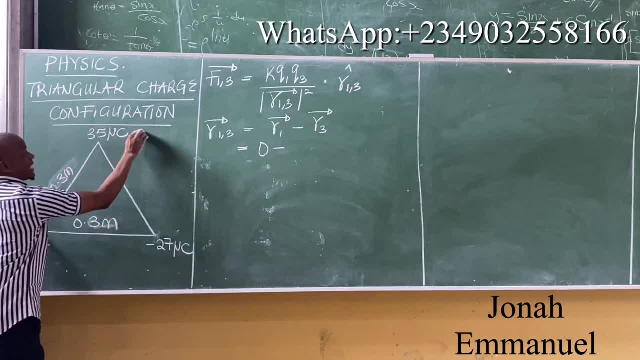 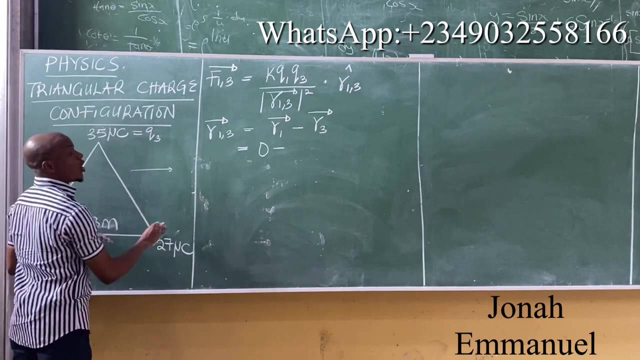 Distance from charge 1,. this is Q3, as we said. Distance from Q1 to Q3, as you can see here is 0.3 meters, But we cannot use this one here At your level. in vectors you only move either perfectly horizontally or perfectly vertically. 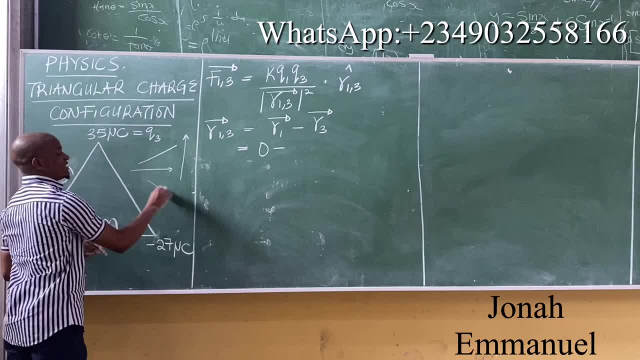 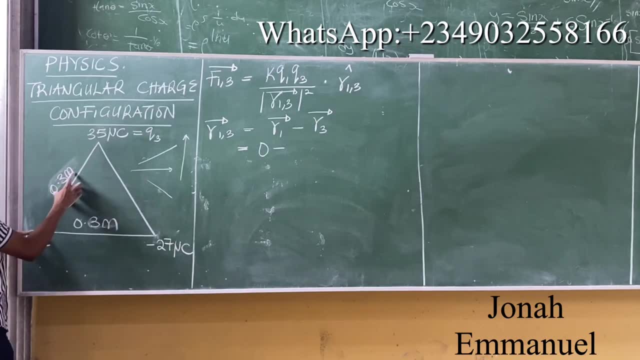 So you cannot move in a diagonal way like this. two are now accepted. in other words, distance from q1 to q3, as you can see, here is actually 0.3 meter, but we cannot use this value recently, because this one here is not perfectly vertical neither. 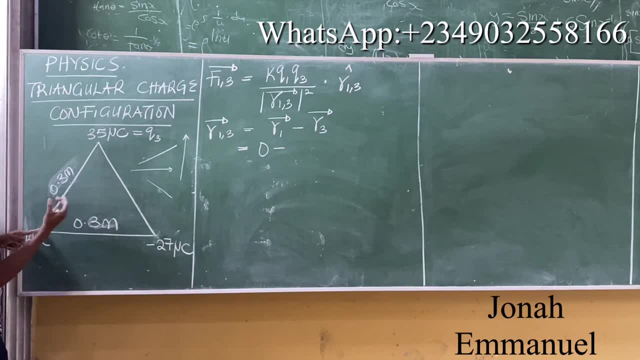 is it perfectly horizontal. my task now be to carve out a distance from here to this way in terms of x and y. and how do i do that? it's as easy as from here. divide this value into this. so, instead of moving from here to here 0.3 straight, you move from here to this point first. 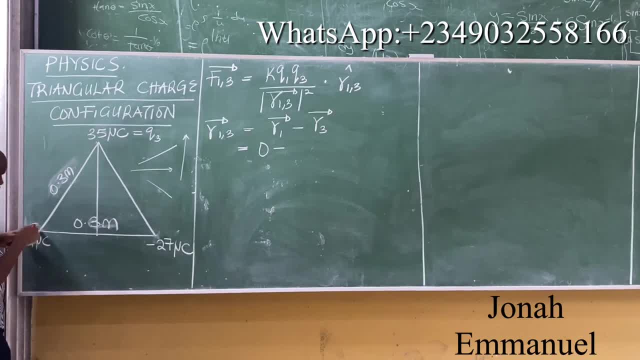 then, from here to this point, when i hit q1 and q2, i do not have to divide this. why? because this time between q1 and q2, as you can see here, is perfectly horizontal, so i don't bother. but when it now comes to q1 and q3, distance here is neither perfectly horizontal or vertical. 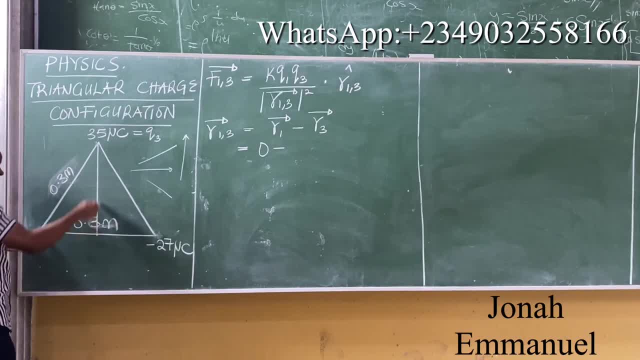 so i have to create the distance from here this way and then this way. so i'm moving this way and this way. now, here's what we know. we know that from here to here is 0.3. if i divide this into three equal halves from here, you see what there: 0.15. so i'm having 0.15 meters as from here. 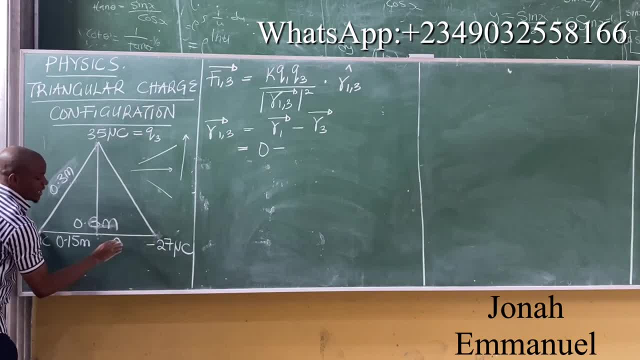 to there. of course, from here to there also becomes 0.15 meters. so this to give you 0.3, that's one, that's one next up. let's get this distance here. we can get this one here using pi kak ross theory, because if i look at this top straight, i can see this. you can see something. 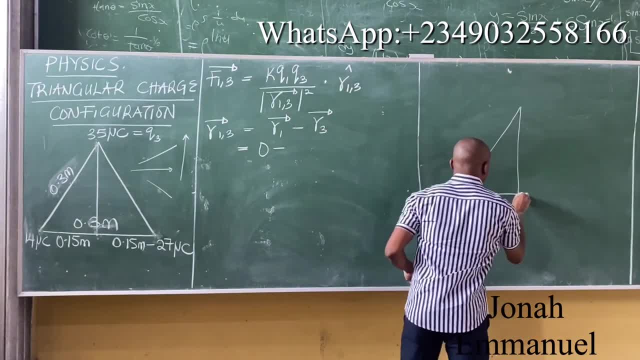 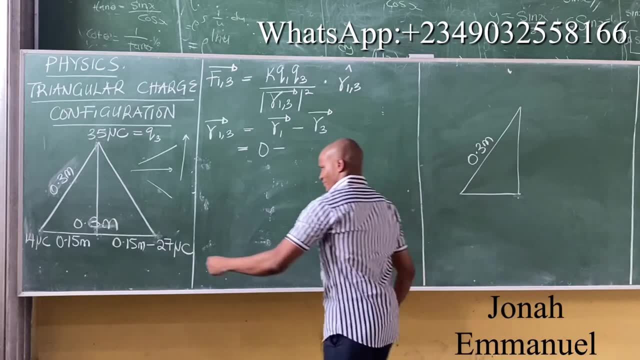 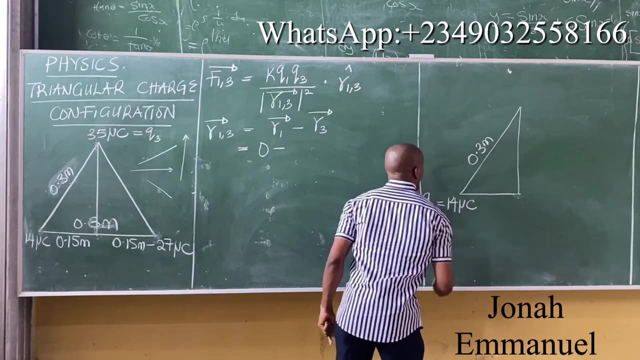 of this nature, this one, this and this, such that we said from here to here is 0.3 meters. i'm having 0.3 meters. at this point, i have q1 being equal to 14 microcoli. at this point, i have 35. 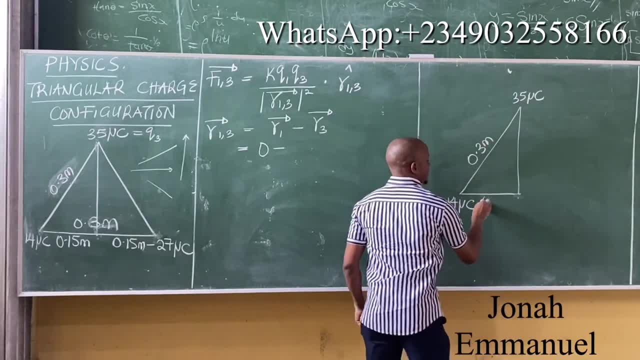 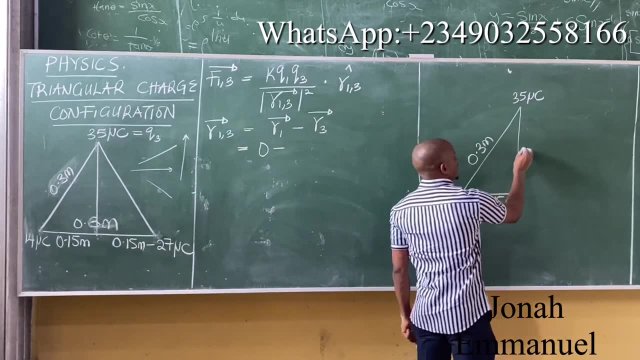 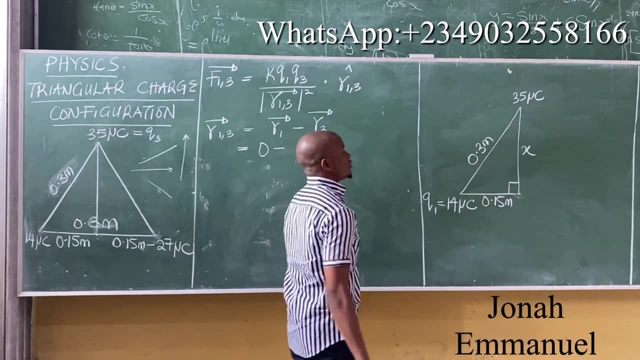 microcoli. we said from here to here is 0.15 meters. that's half of this. my task now is to find this distance x. so how to work with pythagoras theory, since this is what's called a right-handed triangle. so from pythagoras theory it states that the square of the hypotenuse. so here's my hypotenuse. 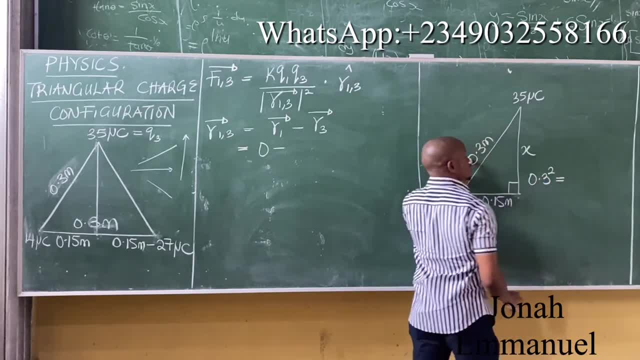 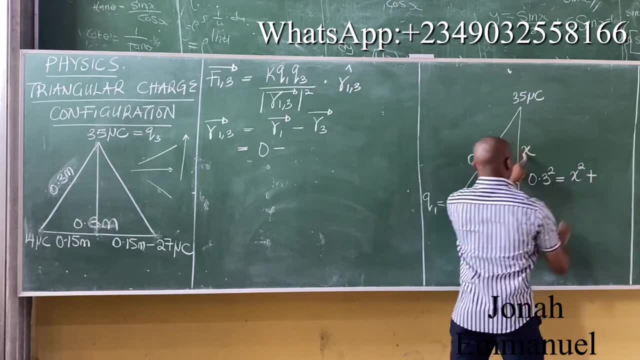 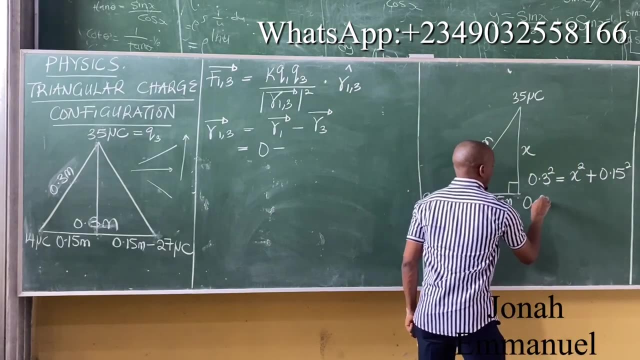 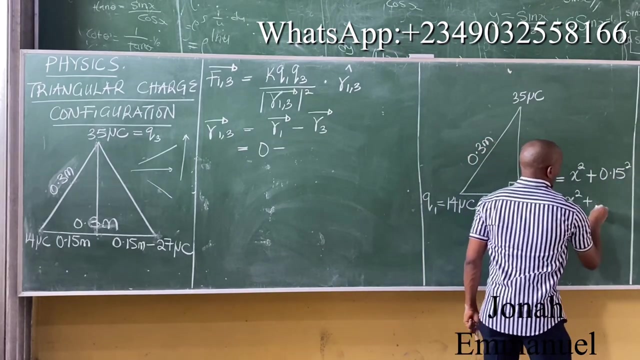 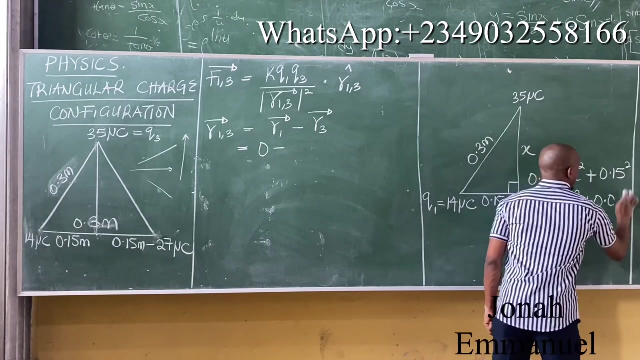 that means 0.3 squared is equal to the sum of the square of the other two sides, to become x squared plus this side here, 0.15 squared. what do you have here? 0.09, yeah, is equal to x squared plus zero point. what? three, five, three five, one, two five, zero point, zero, two, five. so i have this. 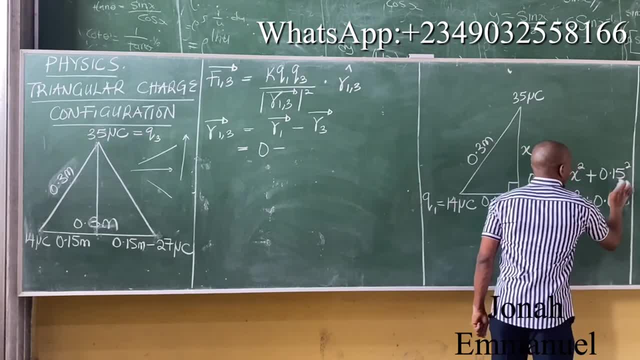 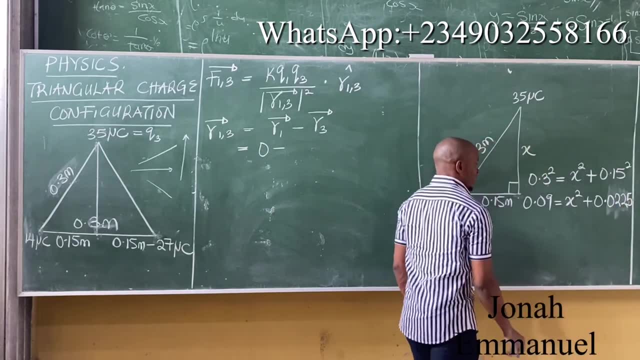 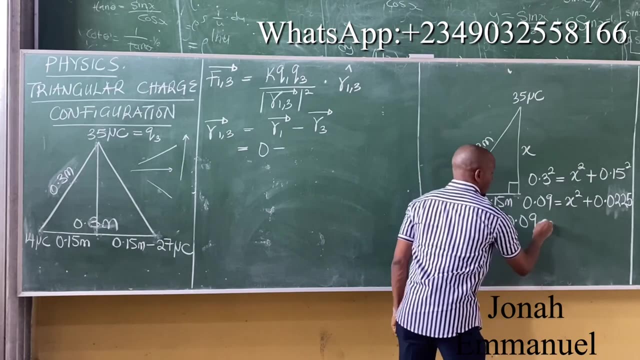 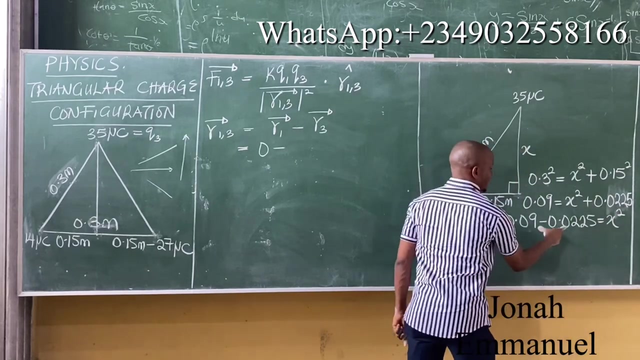 zero point two, two, five. zero point zero, two, two, five. so i have this next tax: bring this manual out there to become zero point zero nine. this, my concept, becomes negative. minus zero point zero two, two five is equal to x squared. give me different. what do you get there? zero point zero, six, seven, five. 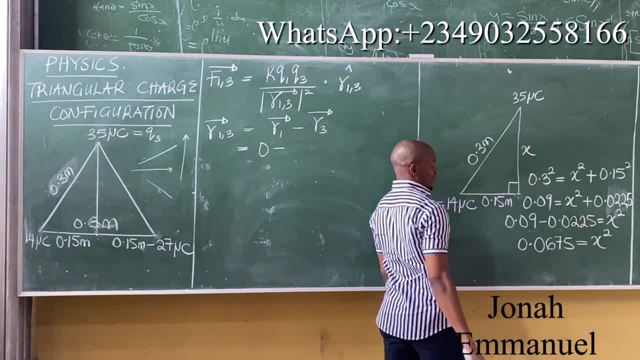 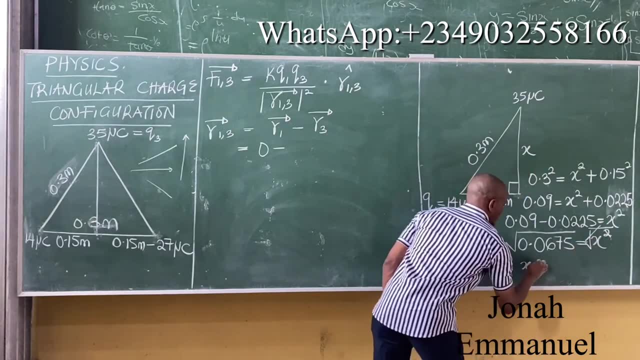 is equal to x squared. To get x, just repeat: x squared, x squared, yeah, x squared, yeah. This cancels this. So x is equal to what do you have there? 0.. 2, 6.. 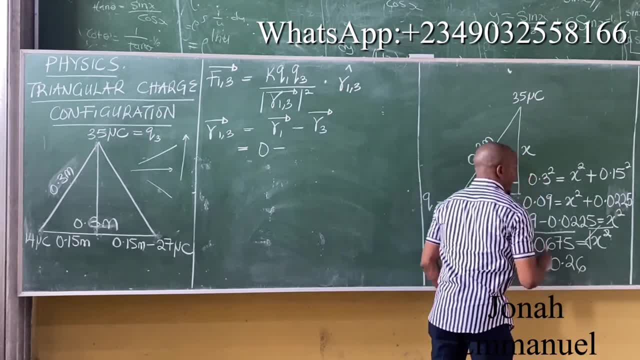 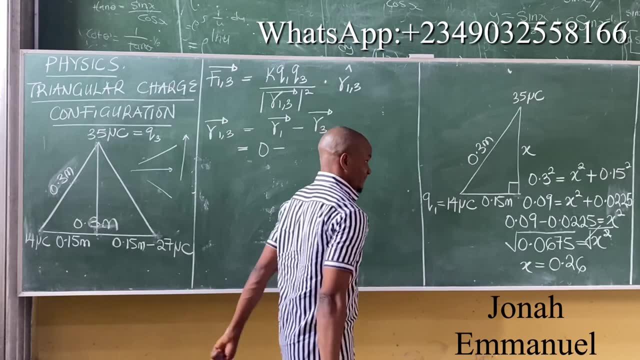 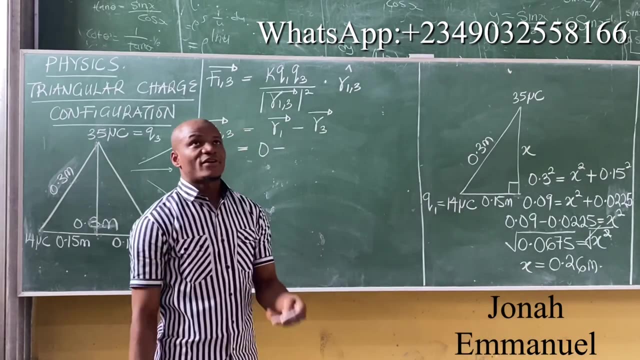 Just 2, 6.. Okay, 0.2.. 5, 9.. Do you have to resume it? Do you have to resume it? Okay, 0.26 meters. I think I would advise you not to resume it. Use 5, 9.. 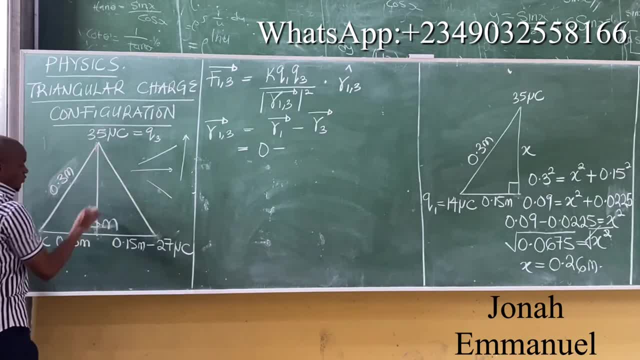 But 2, 6 is still okay. That is from here to here. this one here, in fact, don't have to resume it, Do it by me. Oh, come on, do it on 2, 6.. 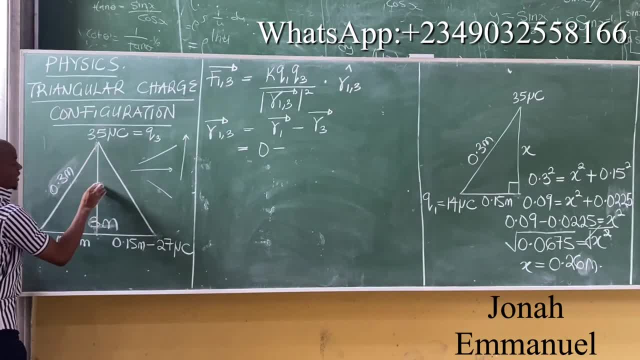 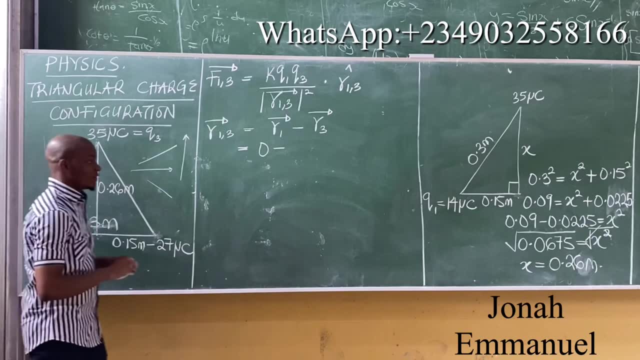 So here now becomes this. distance becomes 0.26 meters. Right, This becomes 0.26.. Later, Alright, So look at this When you are from the top. we are showing what a shelf is like. See, we are shelving. 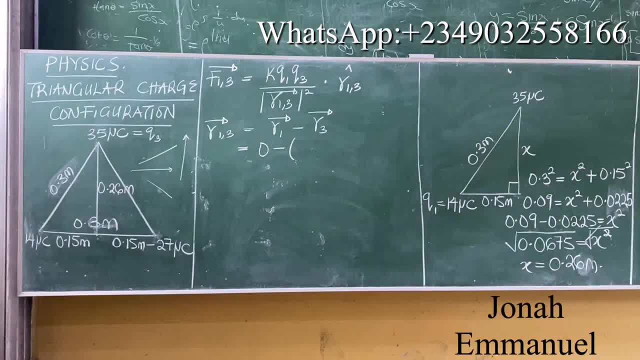 Move. Alright, Let's get R1, please. So look at this. So here is my R1.. Here is R3.. I am moving from R1 to R3.. Please always watch direction. This is your partition coordinate. 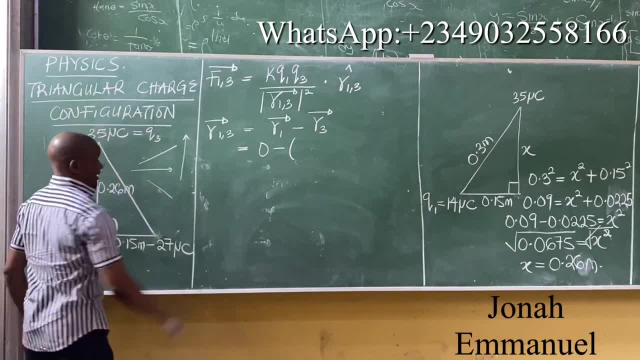 You said: here is cost of the product. This is your R1.. This is your R2.. This is your R3.. This is your R3.. This is your R4.. This is your R5.. This is your R6.. 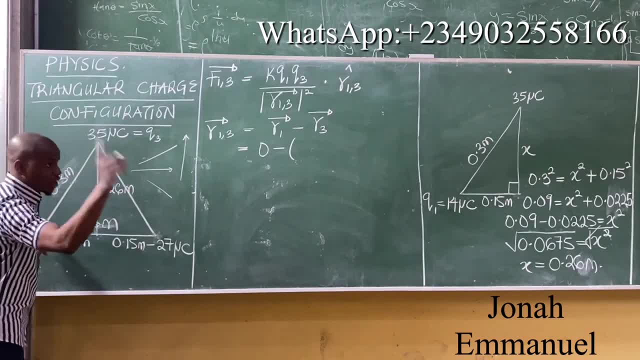 This is your R7.. This is your R8.. This is your R9.. This is your R10.. This is your R11.. This is your R11.. This is your R11.. So R11 is a partition coordinate. You said: here is cost of X. 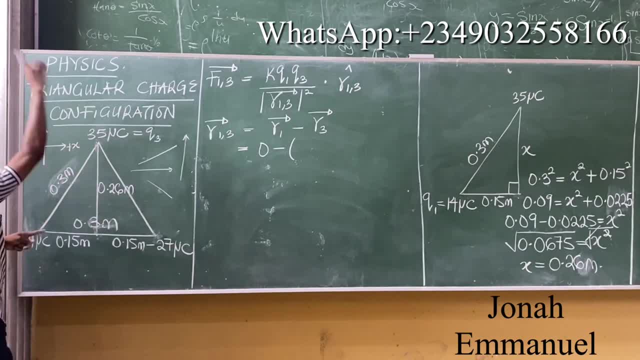 this way: going upwards is cost of Y, So cost of X on the right cost of Y. up I m going upwards. From here I am moving to Q3.. So I am going from here. I would have to move from here. 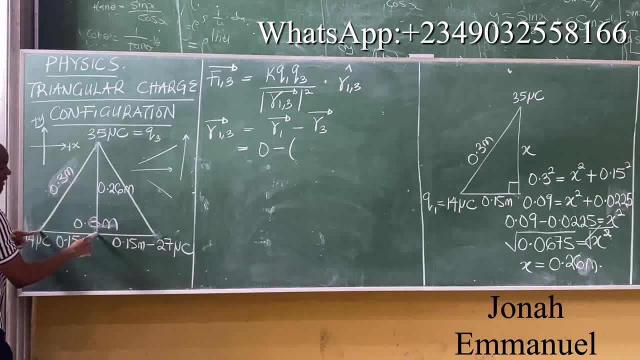 this way first, Then from here this way. So if I move from here to here, this is 0.1. find meters in the X direction That becomes R. So from here to here it's positive because I am going to the right. 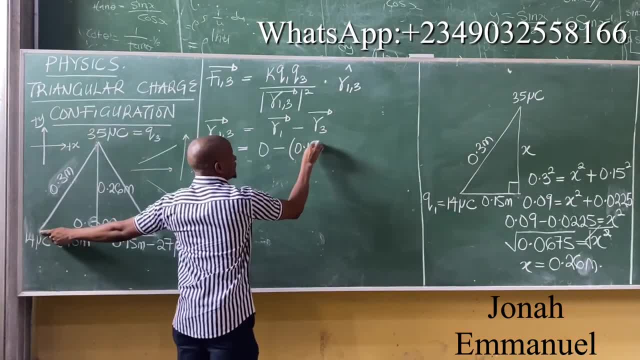 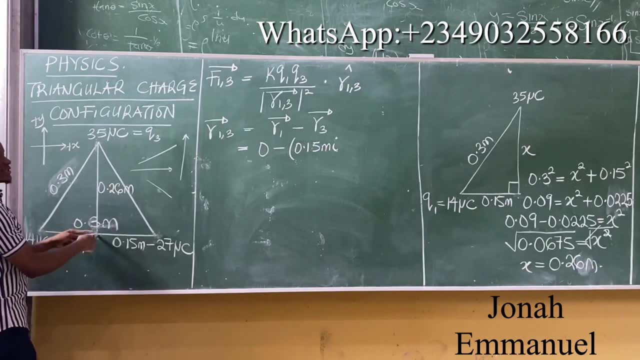 So it becomes 0.1, what you called R1, R2. this way It means the R2.. meters high That becomes from here to this point, But I still have to go upwards. Going upwards is still positive for y, So it becomes plus distance. upwards is from here to here, which is 0.26 meters. 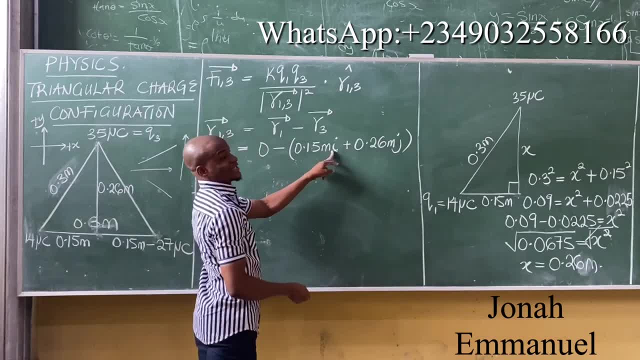 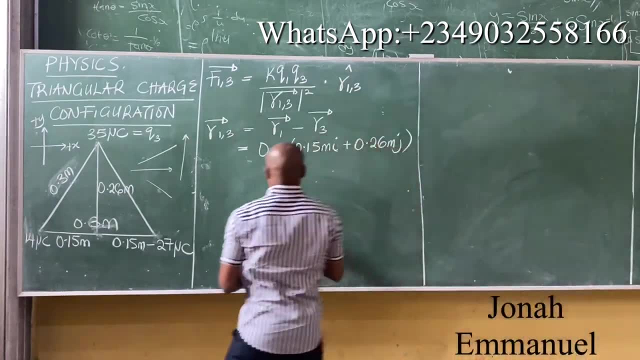 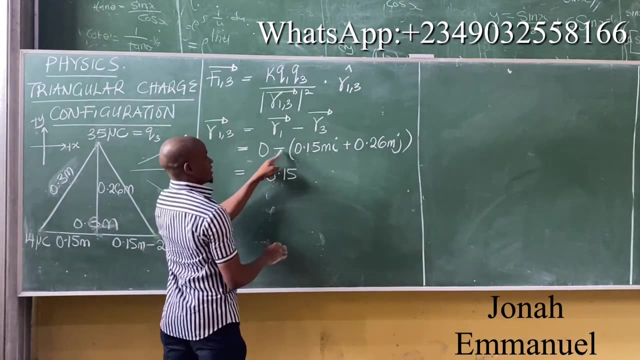 in the what there? J direction. So i for the x direction, j for the y direction and we have this All right. What we have is now equal to. So minus comes here, It gives you minus 0.15.. So this to this. 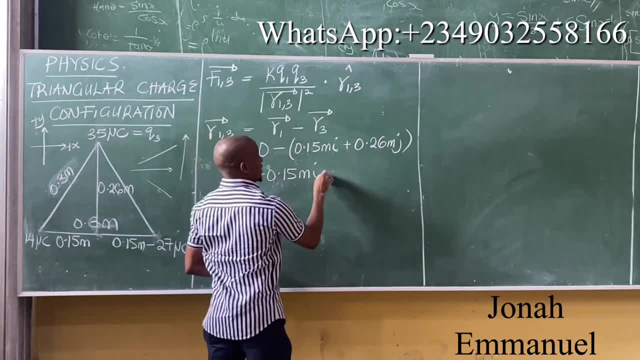 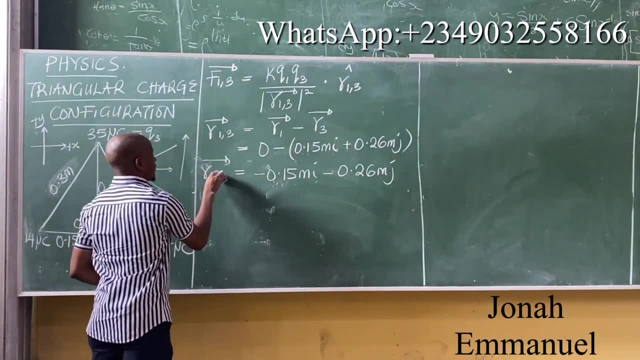 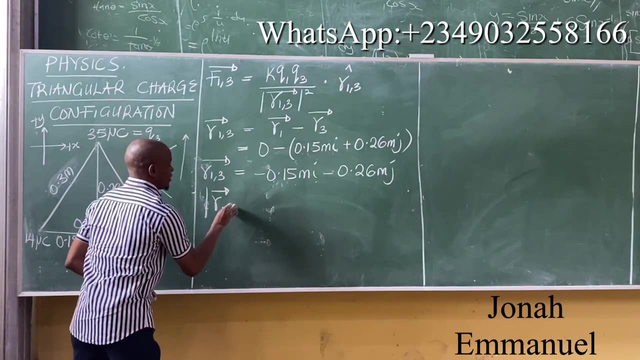 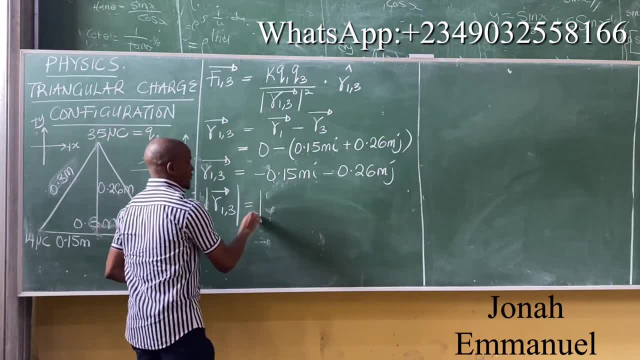 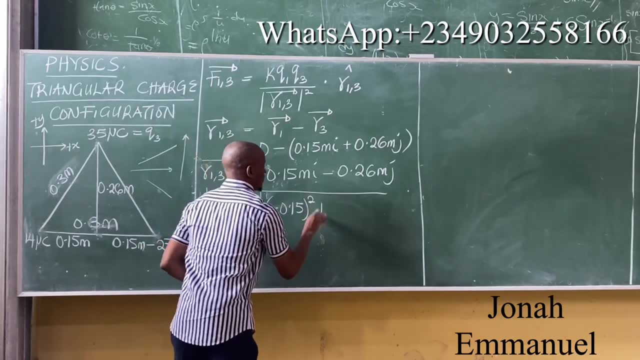 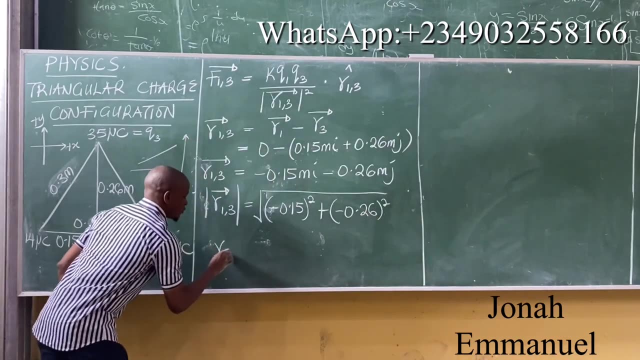 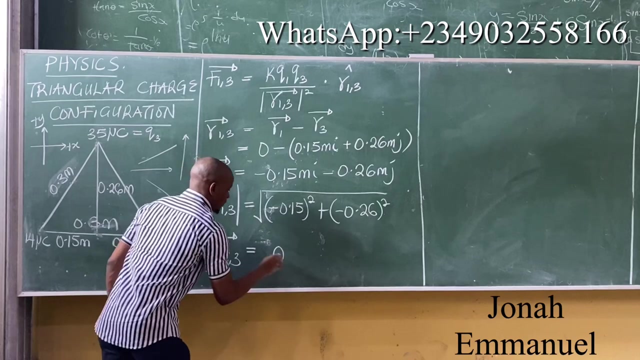 Take the square root of each of them squared, So it becomes the square root of this one first minus 0.15 squared, plus this one next minus 0.26 squared. So we have that r13 is equal to. Please punch and give me final. So what do you have? 0.. what there, Three in what Meters? Observe This magnitude value. 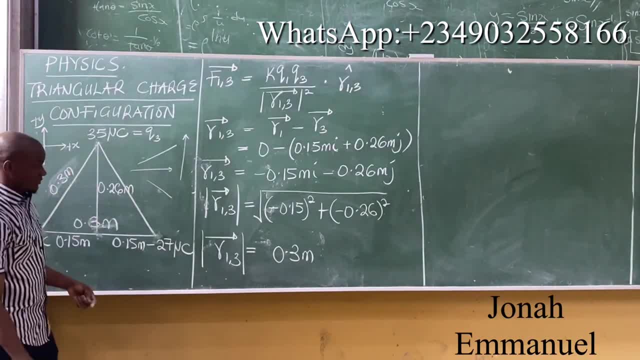 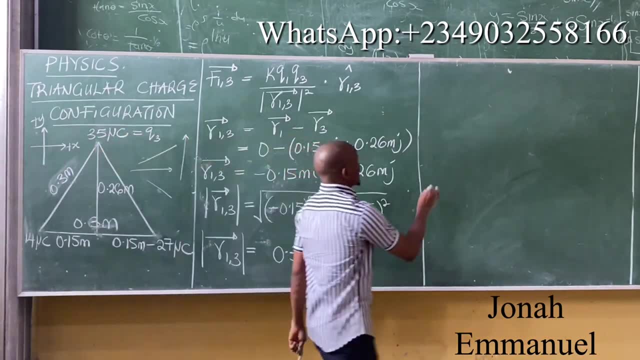 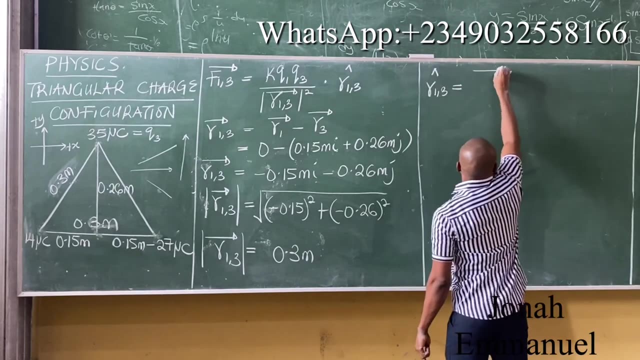 is the same as what you have here. Right, That's how it is. This value will give you same thing as what you have here, So it becomes 0.3 meters. Next task: Get unit vector of r13.. We said the unit vector is equal to. 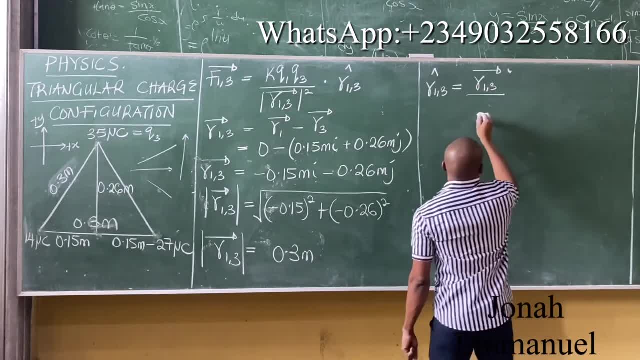 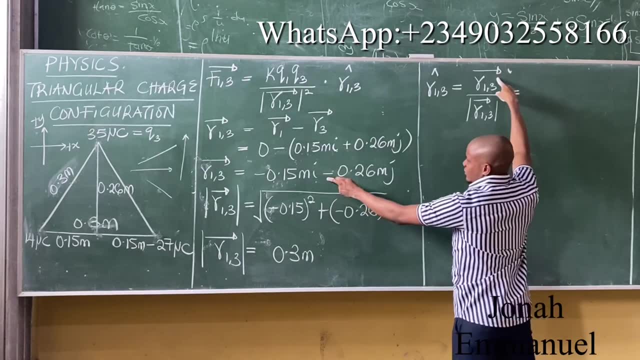 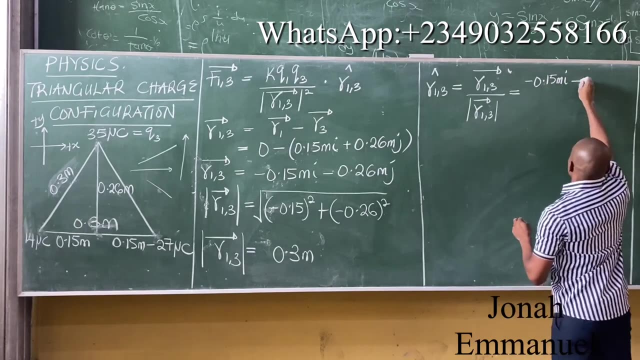 the position vector of r13 all over the magnitude of r13, and that's equal to position vector, is this one, Yeah, And that's minus 0.15 meters high. and then this one there, minus 0.26 meters J, all over this. 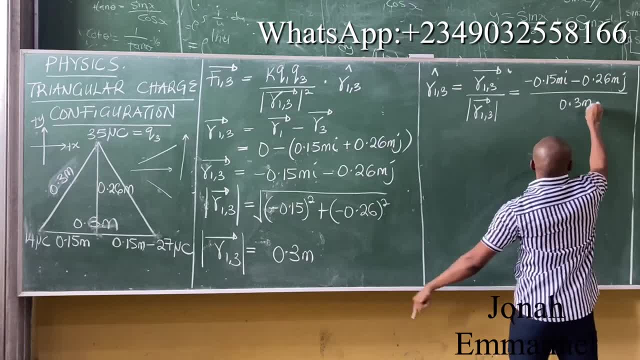 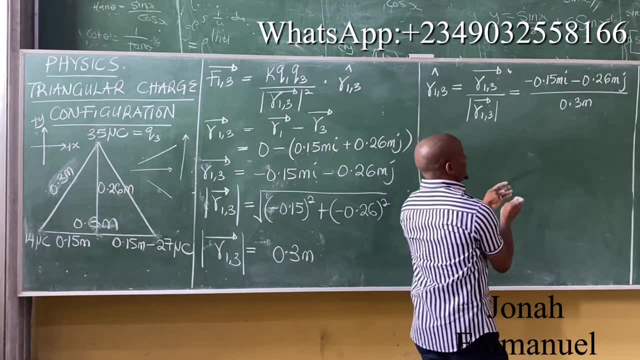 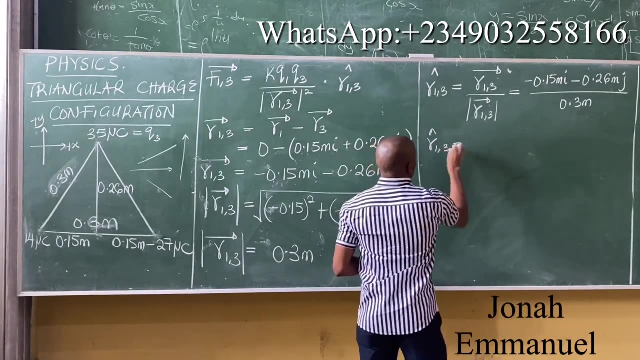 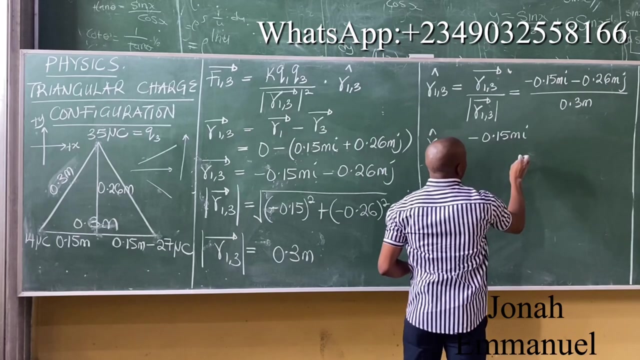 value is this: 0.3 meters. At this point here, at this point here, what you do is this: Take them one by one and simplify, So I'll have that R13 is equal to take this all over this, so it becomes minus 0.15 meters high, all over what I have here: 0.3 meters. Take the. 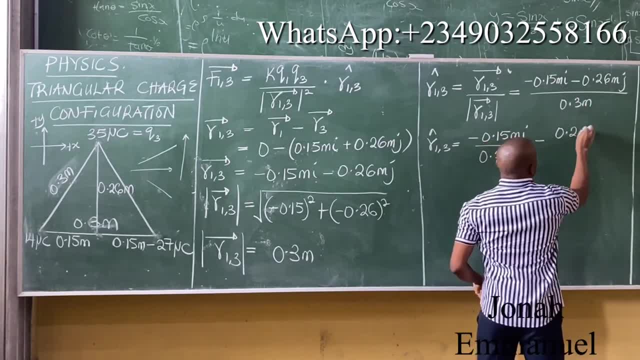 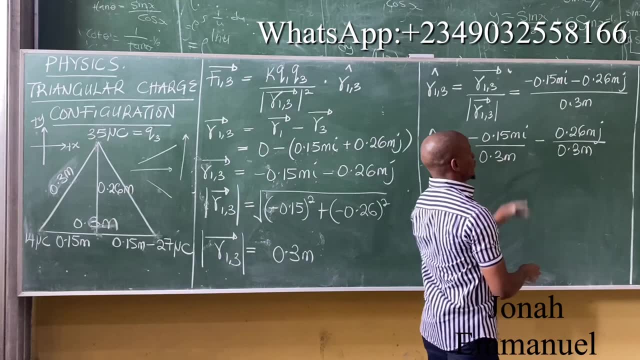 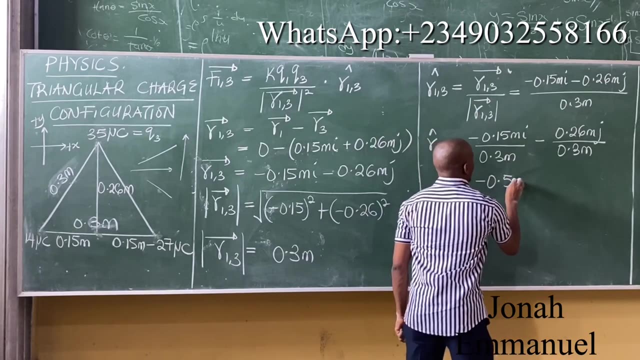 second one: here it becomes minus 0.26 meters J all over what I have here, 0.3 meters. So take them one by one. I have this. Simplify this: what do you get Minus 0.5 meters times? 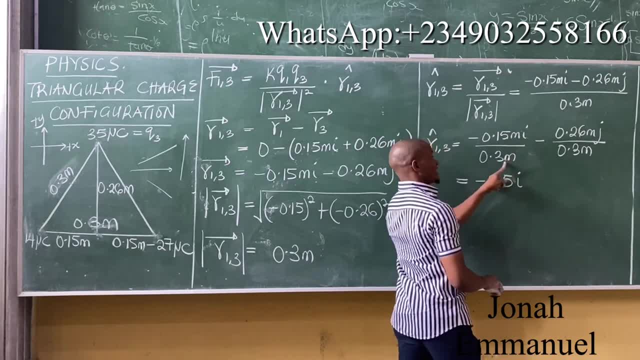 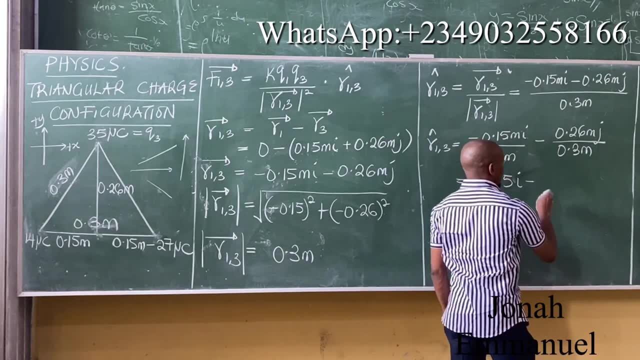 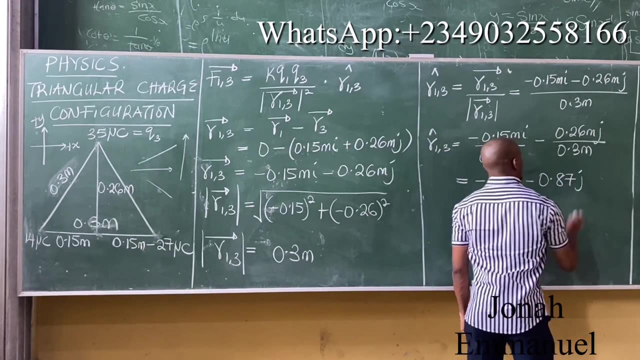 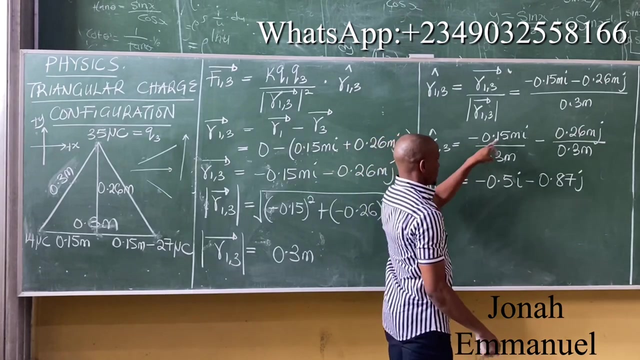 meters And let's go. What's that I so meters times meters. that's I minus what do you have here? Minus 0.867.. Sorry, Minus 0.867.. 0.867, that's 87. what's that? J? This becomes R13.. So I have this right, Minus this by. 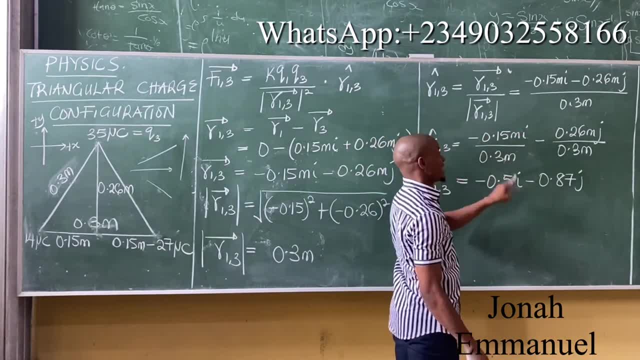 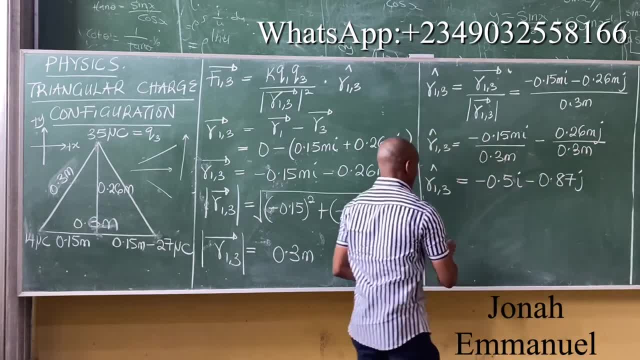 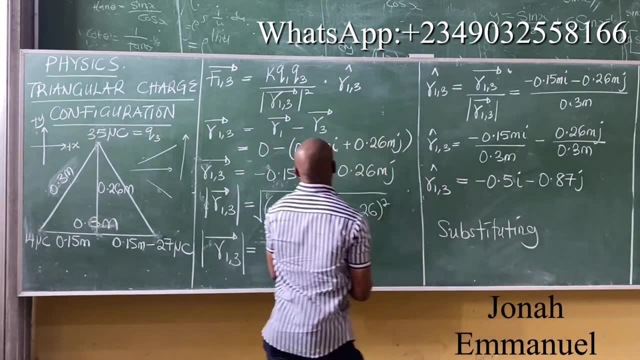 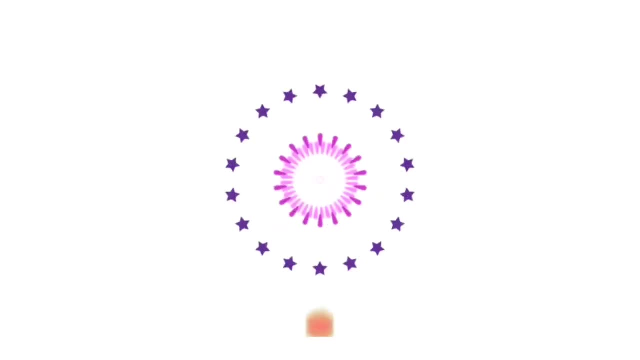 Meters times meters, bring that with J, So I have this Next up. substituting, substituting. So substituting this value back into this equation, All right, Solution of equations. Comparative standards. Substituting. so, if we substitute, is now equal to F1.976. 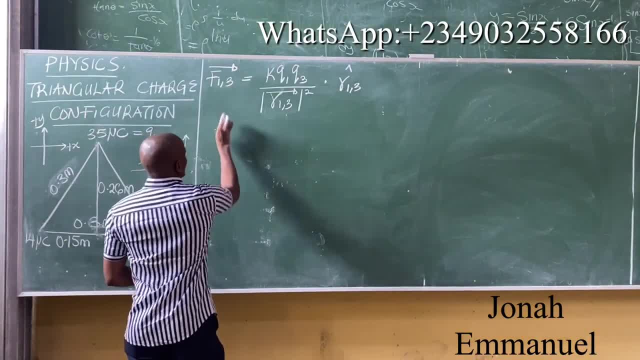 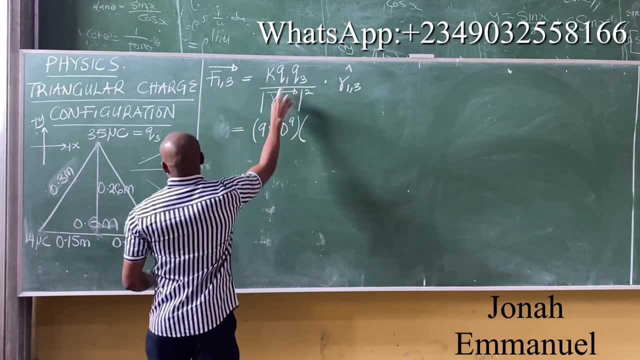 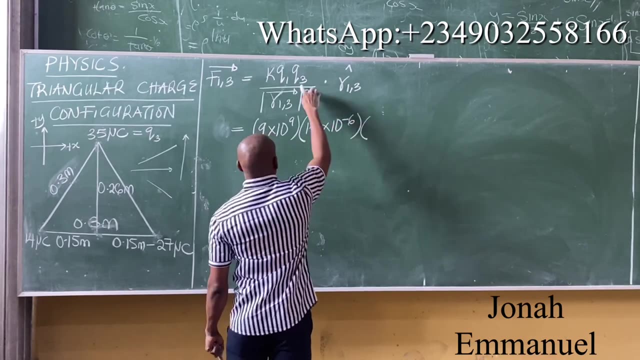 Substituting rest of the equation. Last one again, is equal to K, that's 9 times 10 to the power 9, into Q1, Q1, is this value here 14, this is micro times 10 to the power minus 6, into Q3, Q3 is this one here, that's 35, this is: 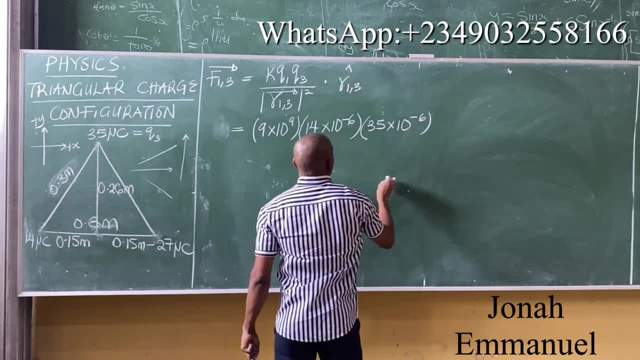 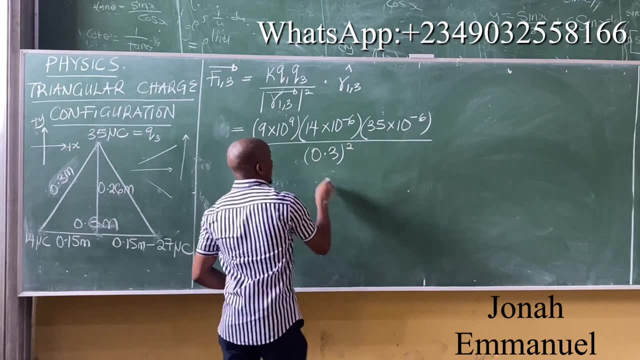 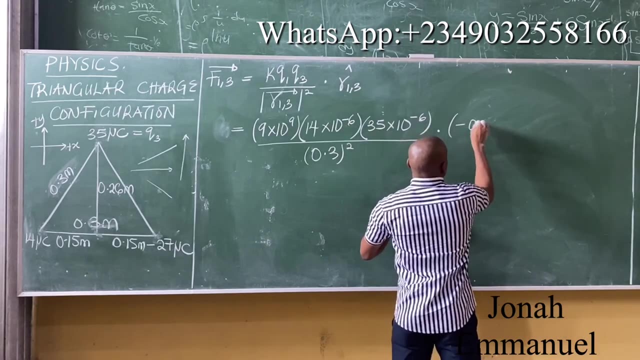 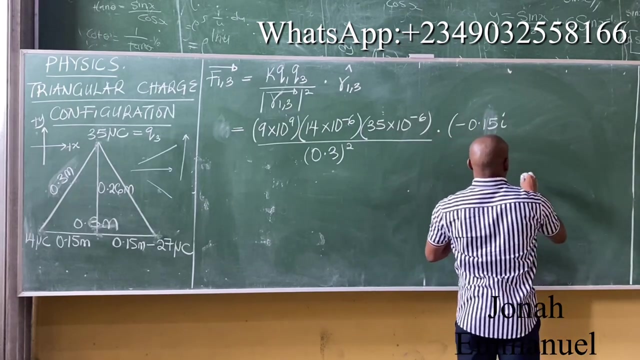 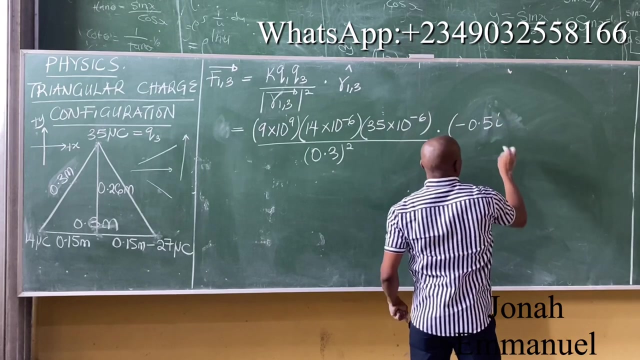 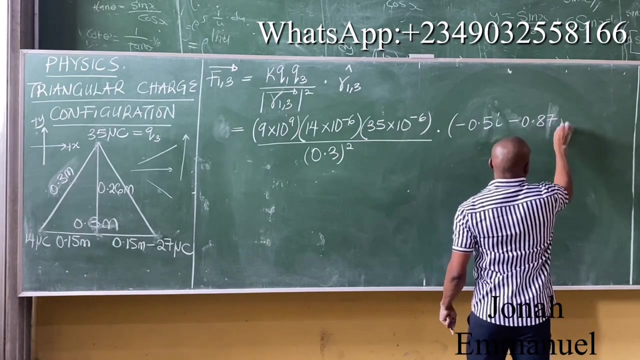 micro 10 to the power minus 6.. All of that, the magnitude as we got was 0.3 R squared multiplied by minus 0.5. I minus 0.5, I minus 0.87, 0.87 J. so we had this. 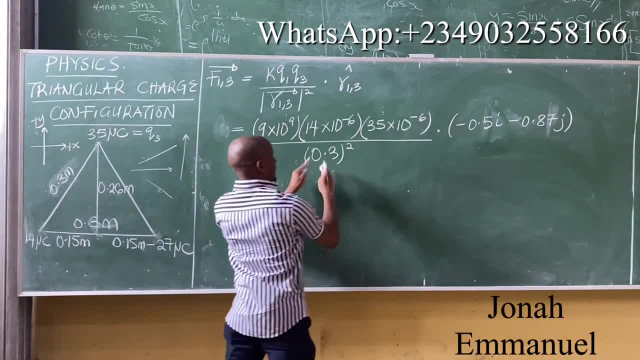 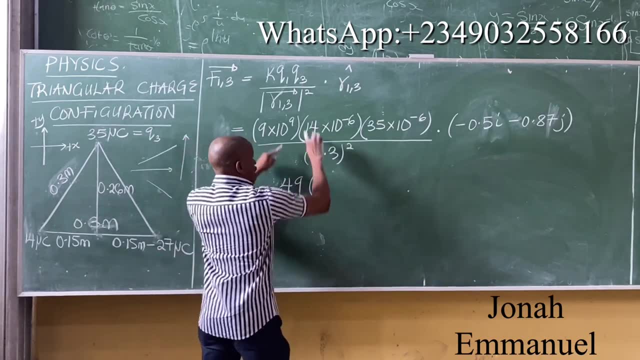 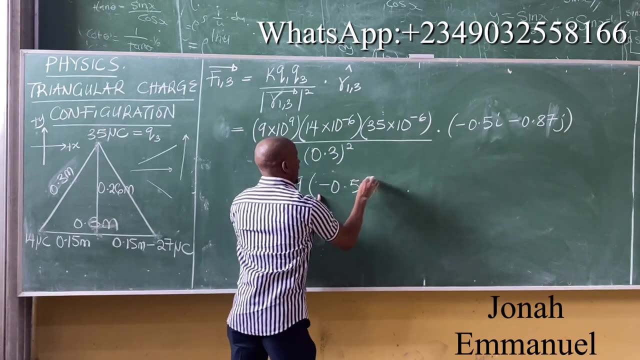 Alright, so that's equal to. please give me all of this value here. what do you have? 49,, 49 dots. okay, So all of this gives 49, into minus 0.3,. this one down 0.5, I, this one next minus 0.87. 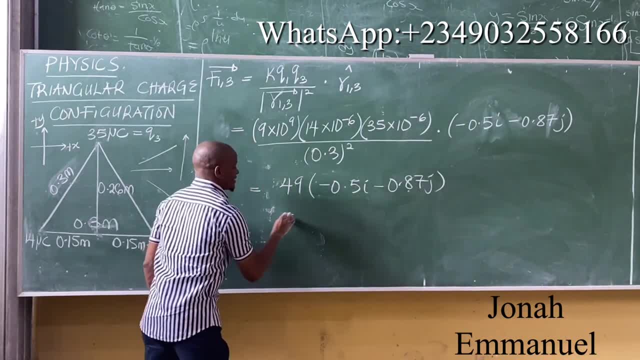 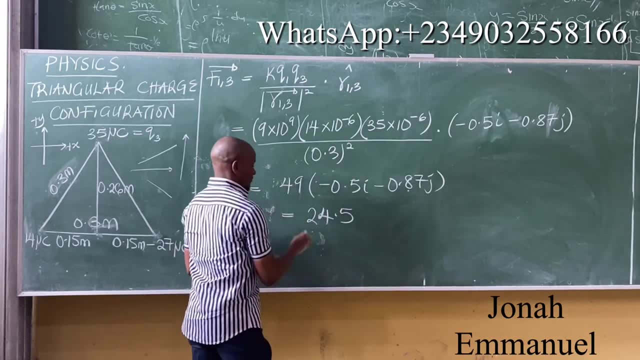 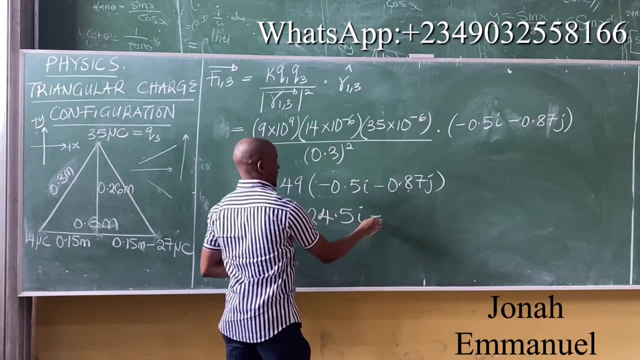 J. So we have this. Please multiply this, this and this. what do you have here? 21,, 24.5, right minus 24.5. I this and this minus. what do you have here? 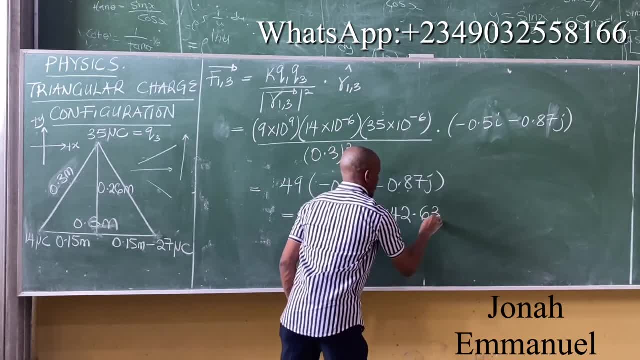 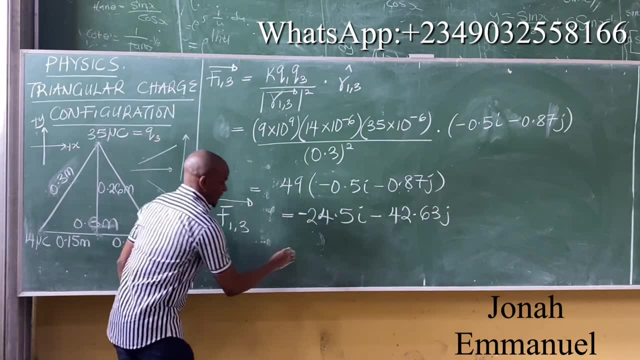 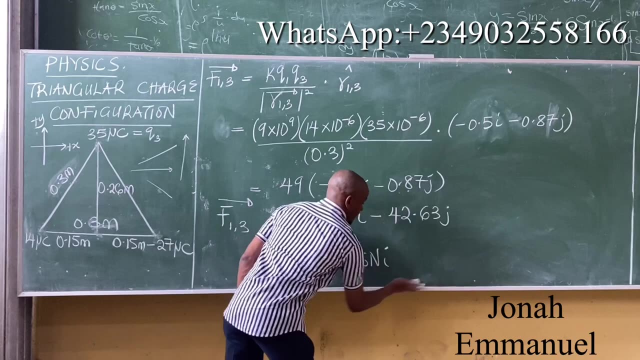 42. 63. 63 J. So since this is a force, that's F13, you have to put the Newton. So that means F13 is equal to minus 24.5 Newton I minus 42.63 Newton J. 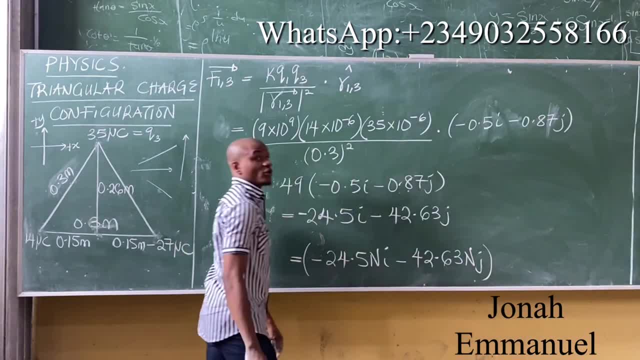 So this becomes the value of F13.. Some authors would prefer to here, to put all of this in brackets and put Newton. Is it the same thing, though? Some authors would put this like this and put Newton outside. Is it the same thing? 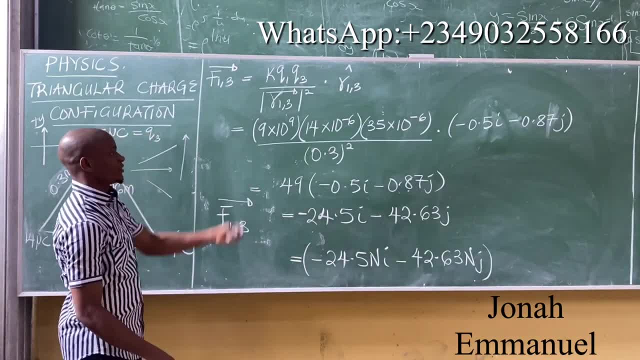 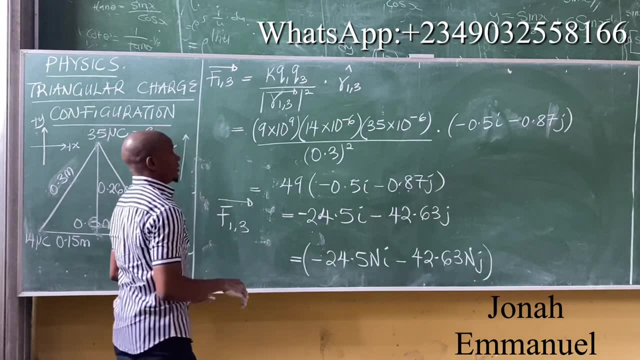 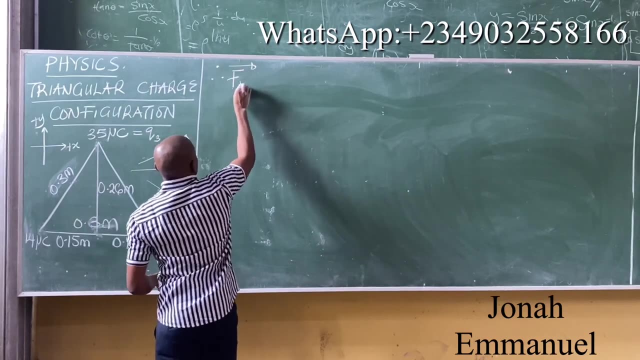 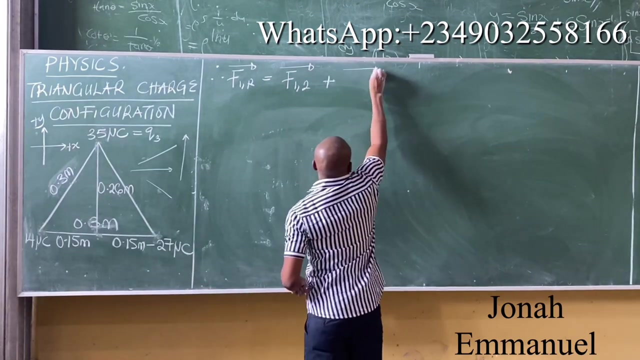 All right, if we have this as F13,, let's get F1 resultant our final value. Let's get F1 resultant our final value. So therefore we have that F1 resultant is equal to F12 plus F13.. 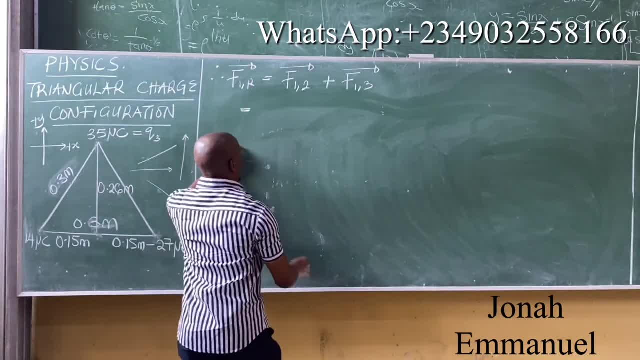 Please recall F12.. What's the value? You have to put that in brackets. Okay, Let's get F12.. You have to count the F12.. We have to put the F12.. How many points do you have there? 27.. 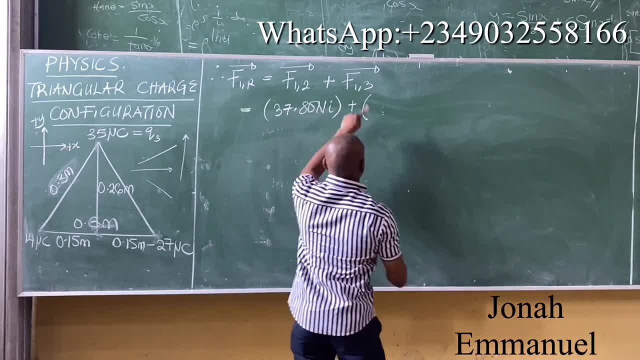 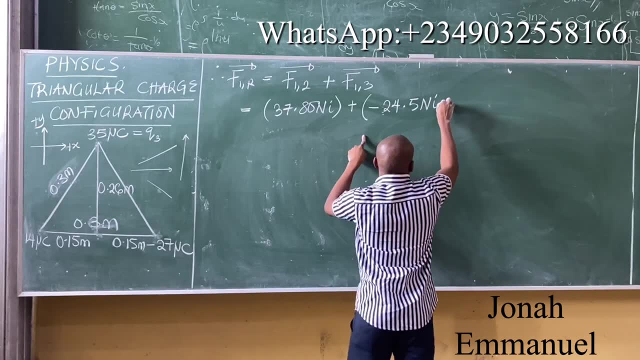 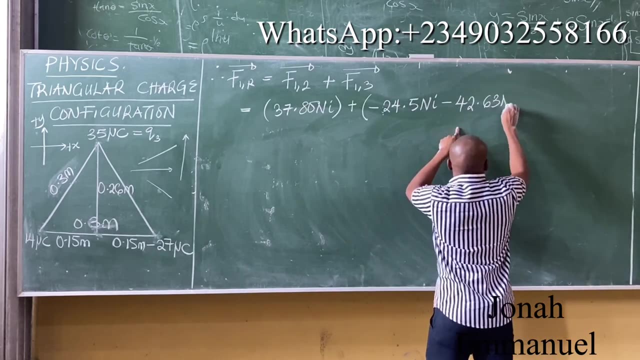 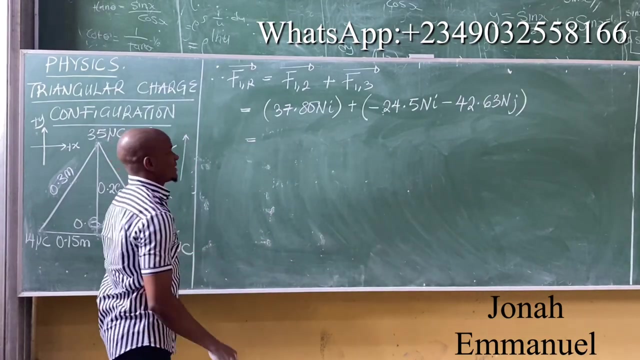 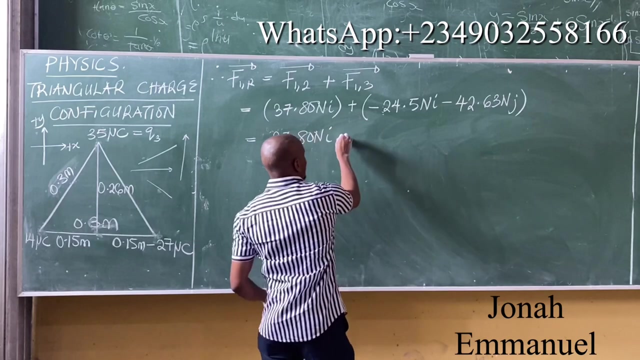 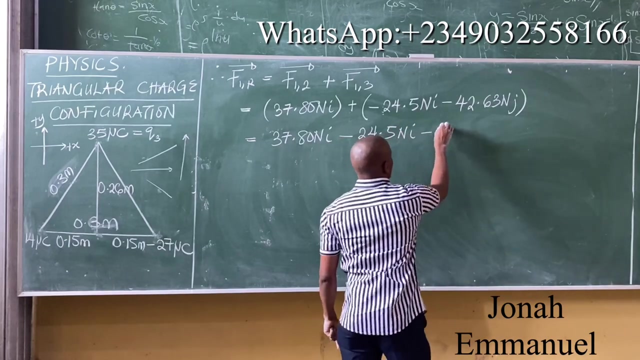 37 points: 8. 0 Newton I plus give me F13.. 24.5 Newton I minus 42.63 Newton J. So recall F1 and F2.. I have these two. I have them Next up. take out the brackets, this becomes 37.80Ni plus minus is minus 24.5Ni plus minus is minus 42.63Ng. 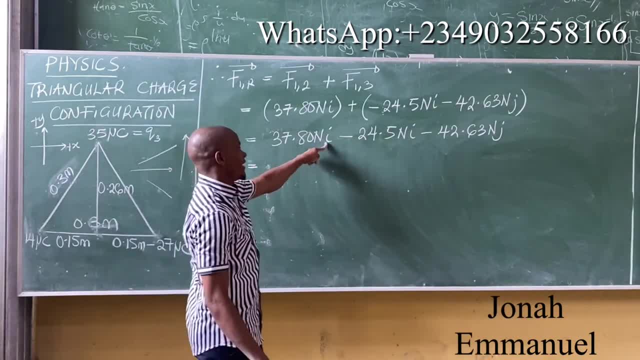 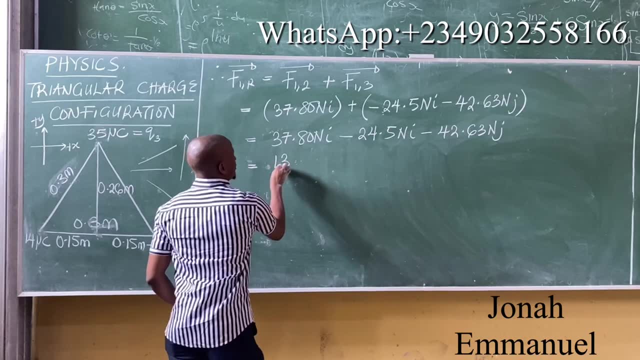 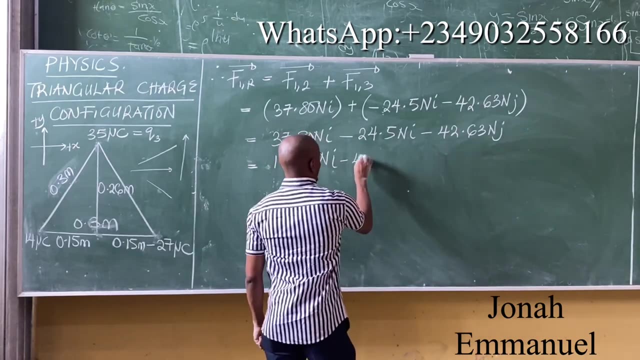 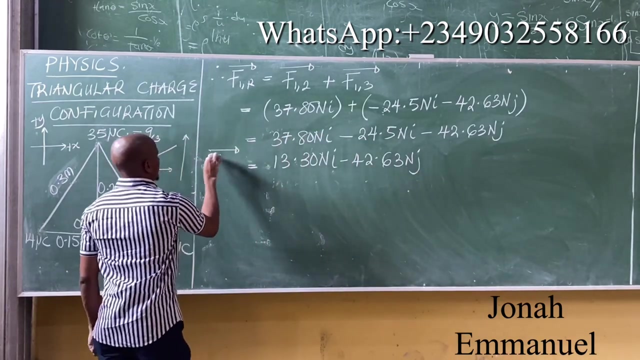 Of course connect like this: this i and this i can subtract because they are like this: Subtract these two. that gives you 13.30Ni. this one here minus 42.63Ng. So this becomes F1 resultant. 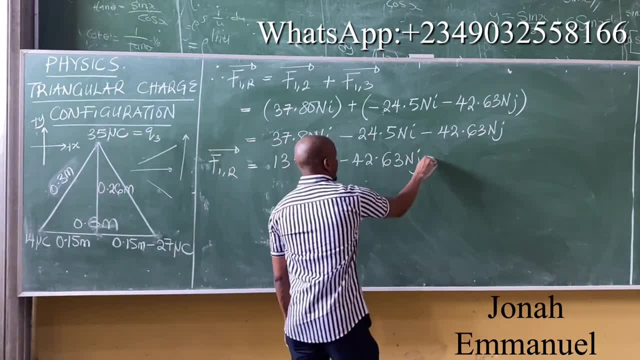 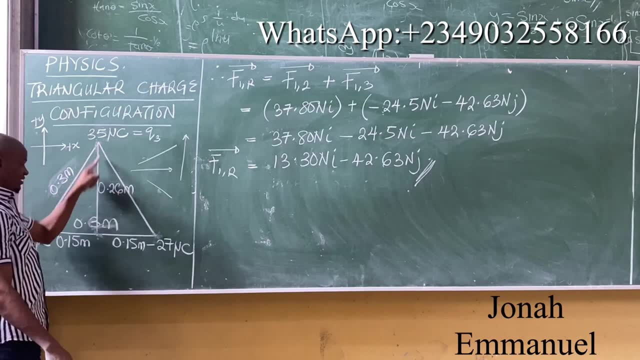 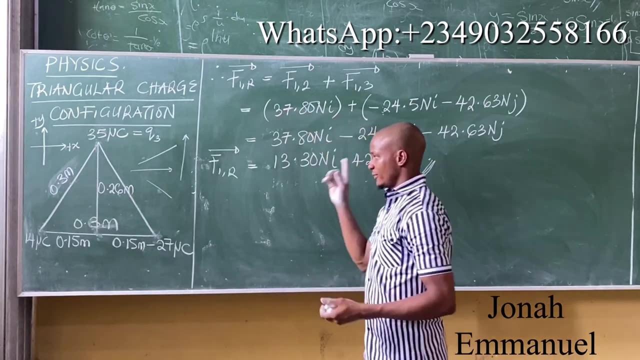 That's how you find resultant force for triangular configuration. I think the only difference there is that for triangular. don't forget we are moving this way, Don't forget this. that's all. That's how you get this much here. That's how you solve this. 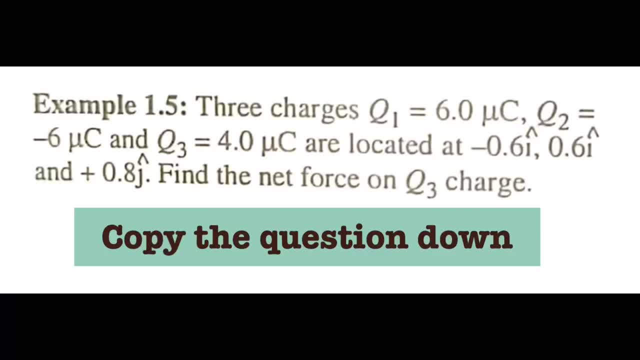 Try this please. Three charges- Q1, equal to 6.0 µC, Q2, equal to minus 6.0 µC and Q3, equal to 4.0 µC- are located at F2.. What is F2?? 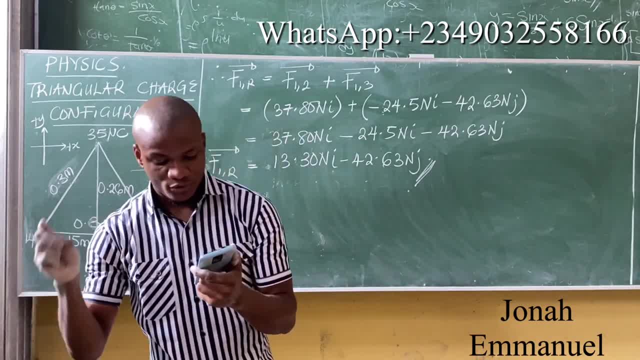 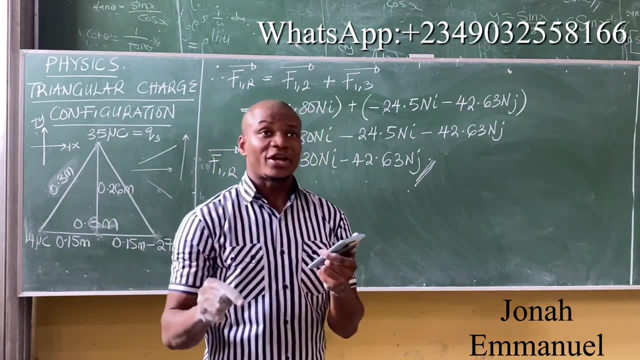 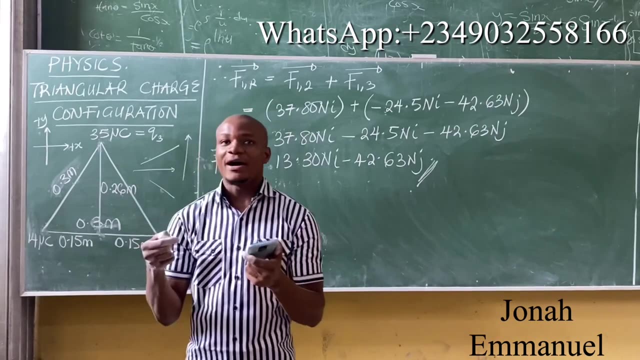 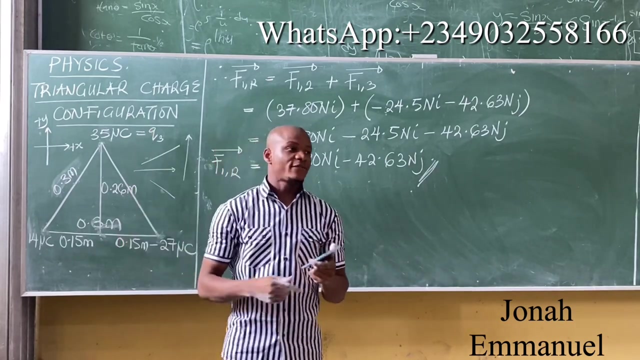 F2 is equal to minus 4.0 µC. Now it is Q3.. Now it is Q4.. So this is equal to minus 3.0 µC, So Q4.. at minus 0.6 i comma, 0.6 i i plus 0.6 0.8 g, find the net cost on q3. that's your question. 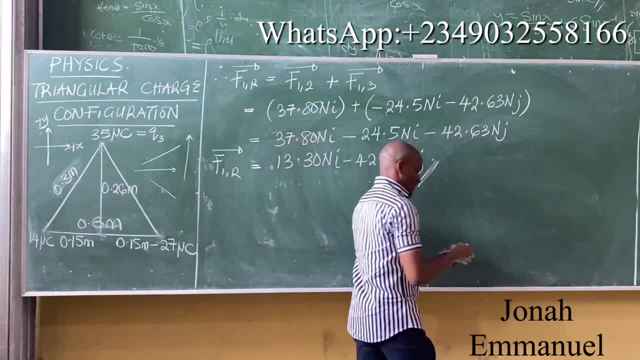 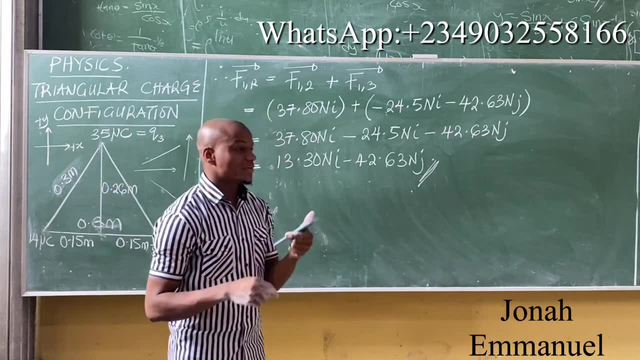 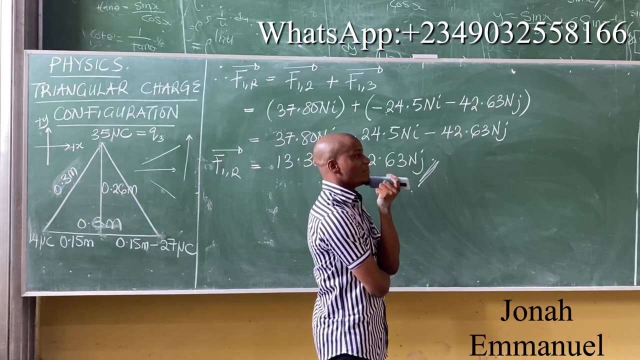 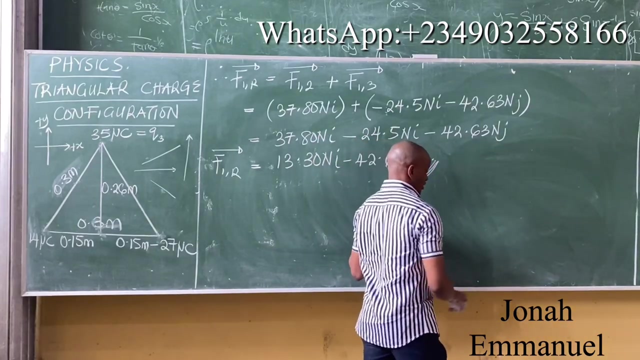 all right. so so here's the thing there. i have three charges there. uh, what's my question? three charges that q1 is 6.0, q2 is minus 6.0, q3 is 4.0. microcoding they said: allocate a little bit of water minus i, minus 0.6 i, plus 0.6 i and plus 0.8. so case one: what we? 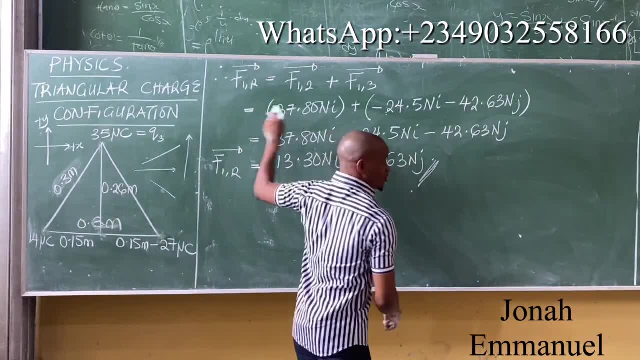 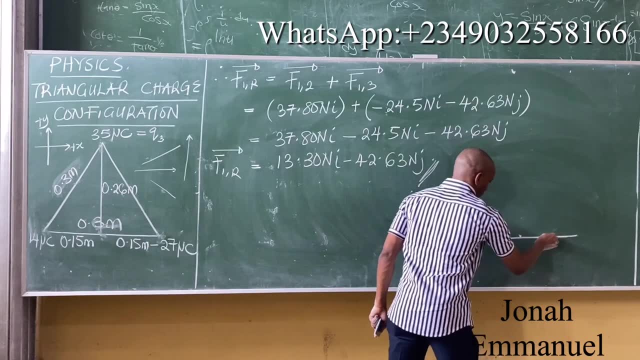 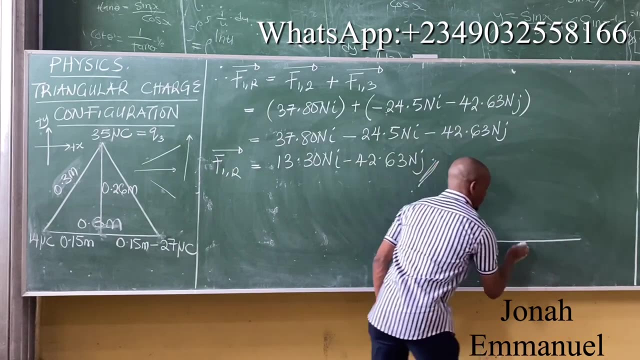 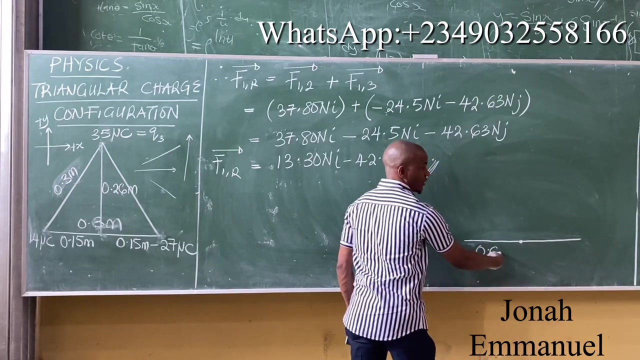 say you have a minus i. that is about a negative region of x, that's minus i. that means i'll have something of this nature. create it. um, sorry, excuse me. so just create a straight line. put the center here. take from here to here as 0.6. 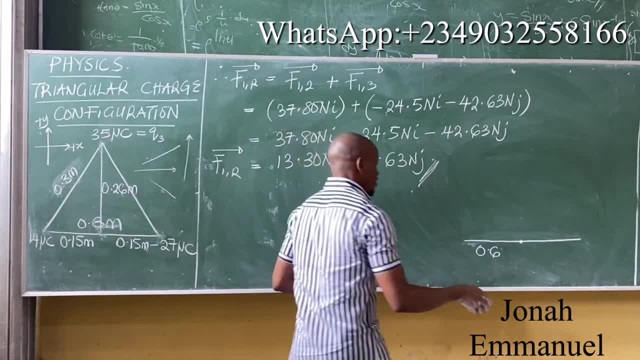 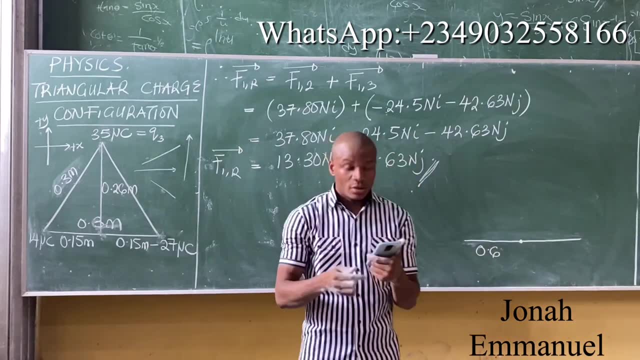 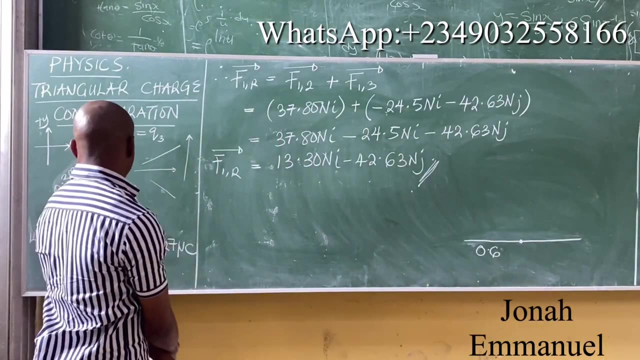 it says this node. it says at minus 0.6. i do i add minus here? listen what you have, listen what you have, what i saw there. um, check your notes. what are you doing here When we get this value? check What would be the sum in here? 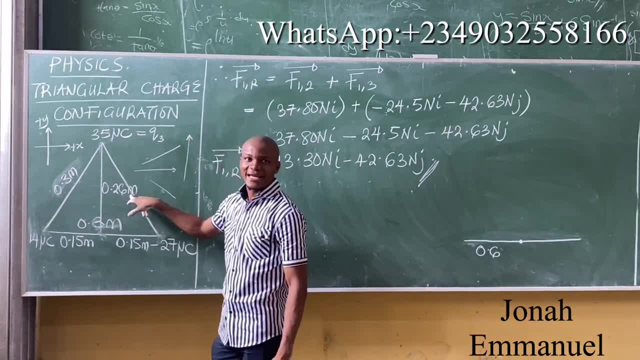 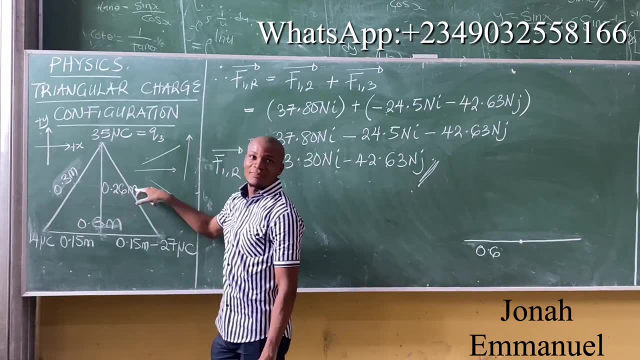 This one was this one: give us about 0.26 meters high, Abhi. check, Check this. We wrote this in our solving check. What would be the unit vector? This: give us plus 0.26 meters high. 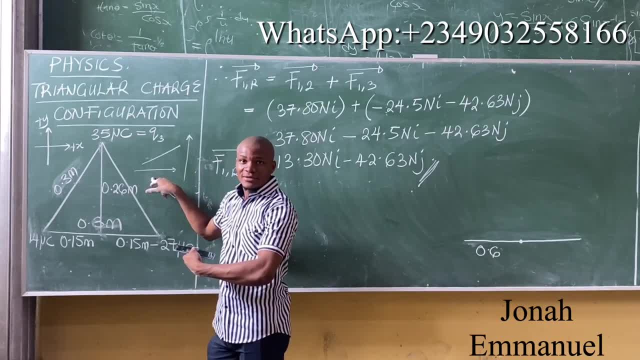 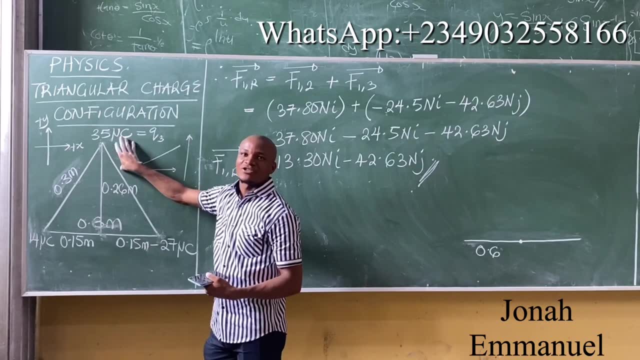 Before we attach minus. Can you see that? Huh, Check your notes. what would be this example? Look for R13.. When we had R1 minus R3. It was zero minus 0.15 meters high Abhi. 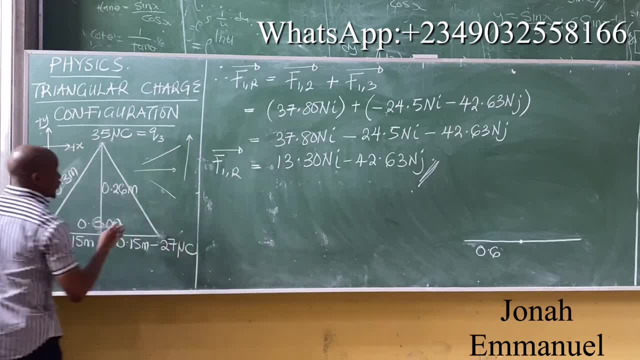 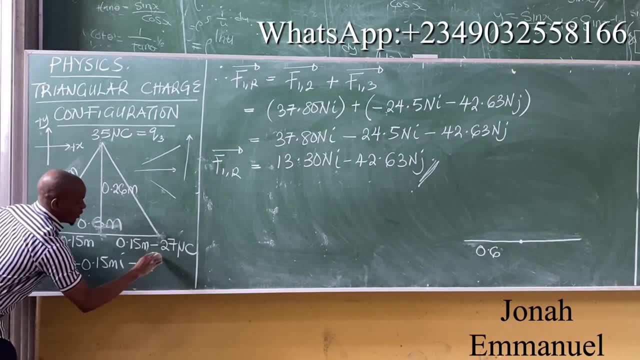 All right. So look at this. please Check R13, R13. give us this: Minus 0.15 meters high, minus 0.26 meters deep. Check this, Abhi. Yes, Now observe something. observe When I was doing my unit vector here. 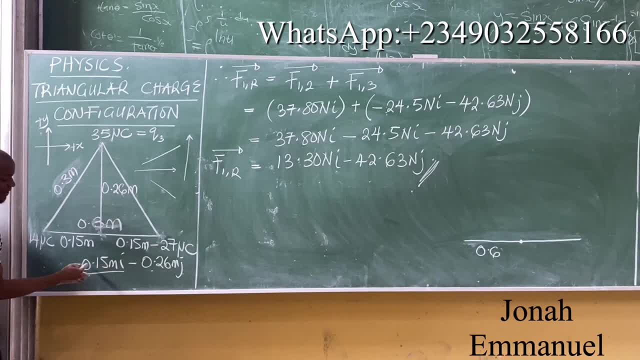 this value was minus 0.15 meters high. Observe that in my diagram there is no minus. there is no I. Minus tells you that it is a negative sign from my point here. negative, I tells you. it lies horizontally the same concept here. 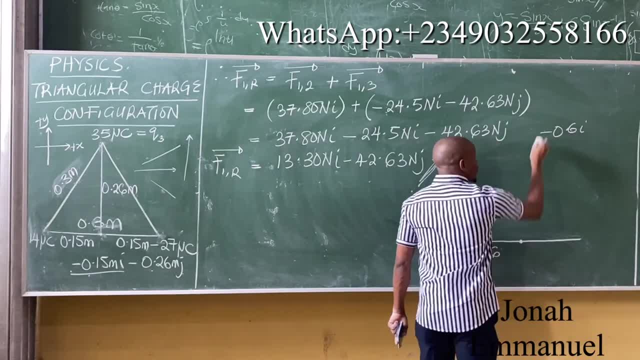 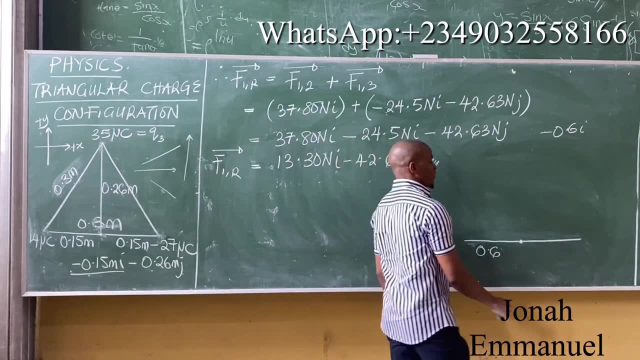 So if you tell you minus 0.6 R. minus means it should be a negative part, I means it's what there horizontally? that's all. Next we now say plus 0.6 R, that's here. The last one now says: plus 0.6 R, that's here. 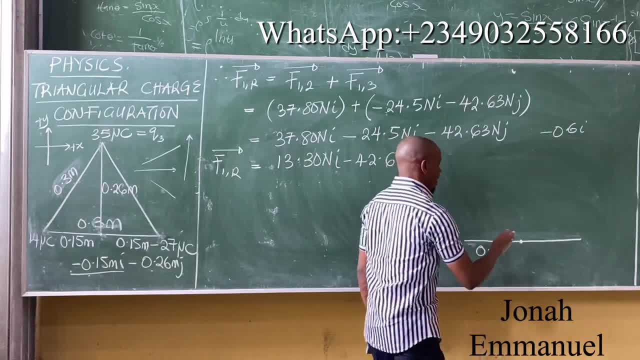 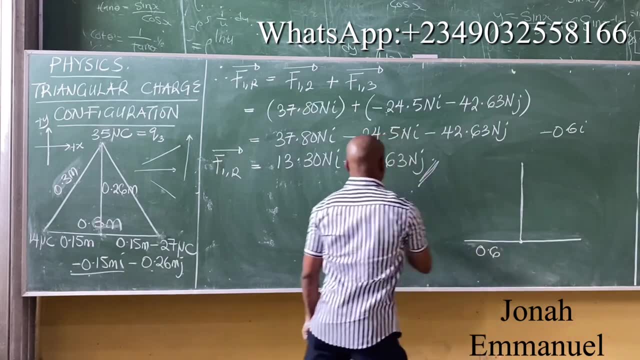 Next, we now say: plus 0.6 R, that's here. Plus 0.1,, plus 0.8g, That will be from here, Go up there. so when you say plus, when you say j, j talks about the vertical axis. 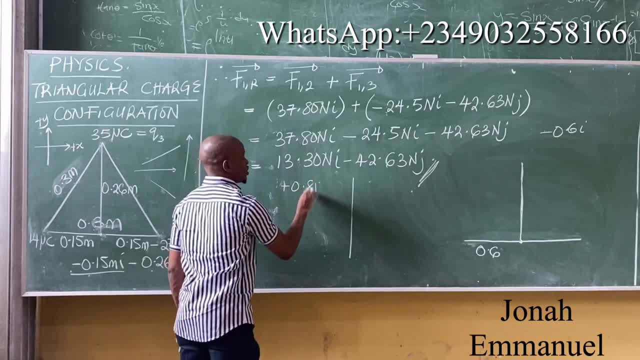 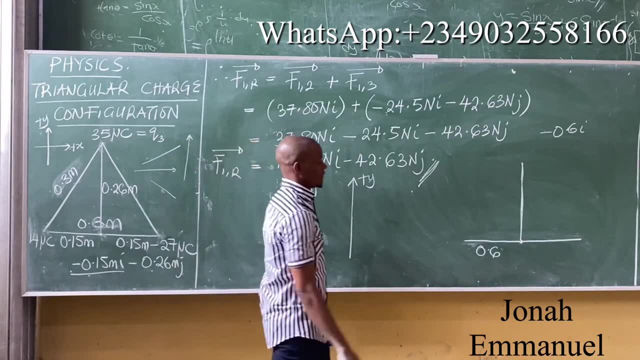 That's j. So if you say plus 0.8, j plus means it's a positive sign of y, so I'm doing upwards, j means it's a vertical direction. So I have this man here as 0.8 meters. 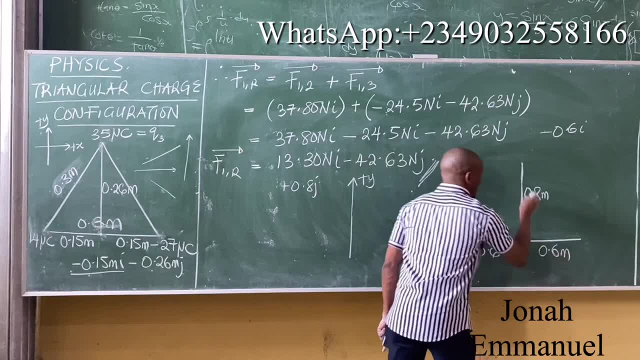 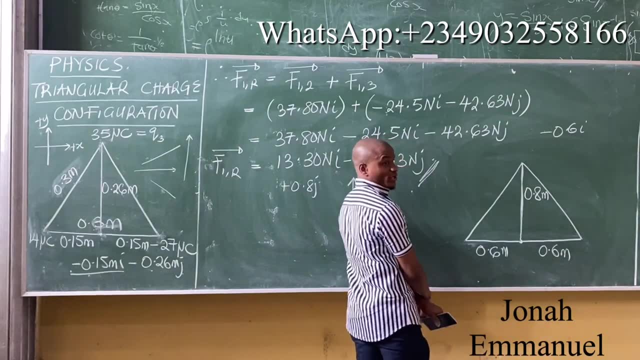 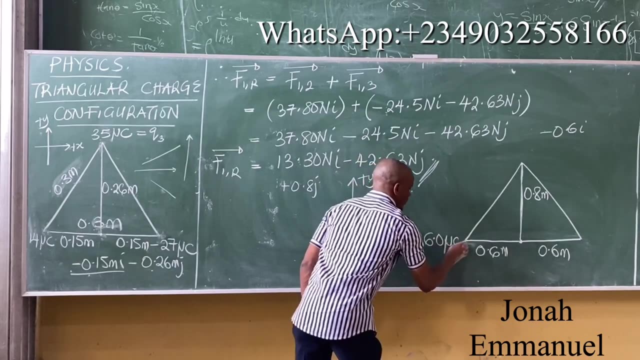 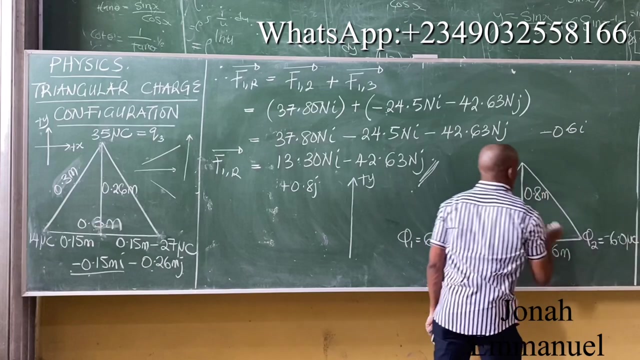 0.6 meters, 0.6 meters meter. so i have this and then this. all right, what's minus eight? no, what was q1? 6.0 microcoli, q2 was there? q2 is what there? minus 6.0 microcoli- q3 is what. 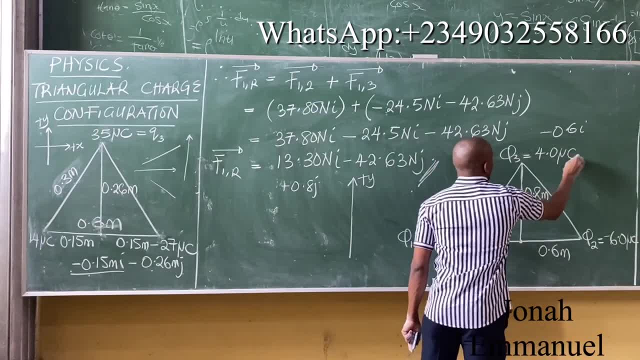 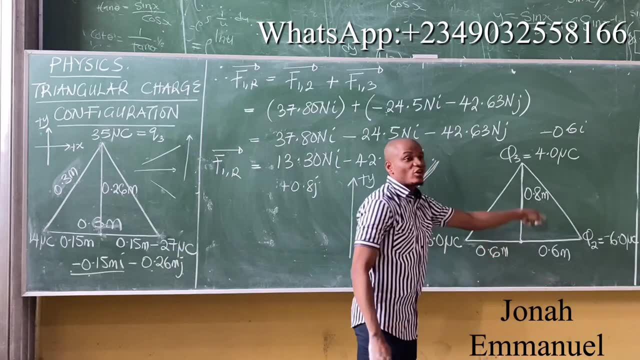 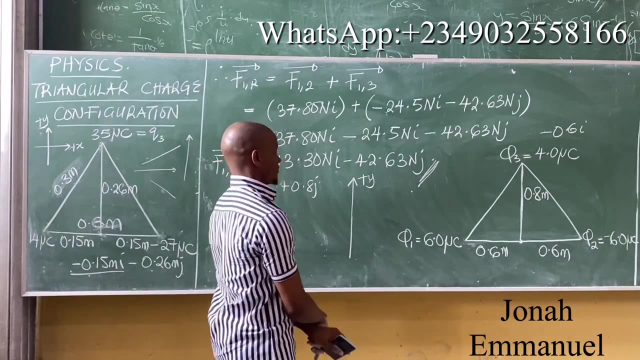 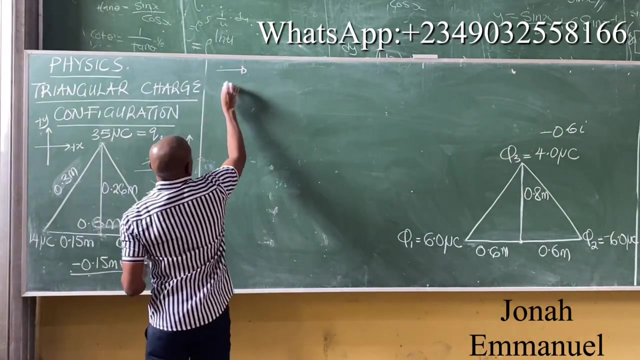 4.0 microcoli. when it comes to the charges in the chart, i'll put in minus in the direction. i can ignore the minus. that's it. so question. uh, i'm not solving this, but we'll now be okay. so check this out please. five arrow, three resultants or the resultant force on the q3 chart. 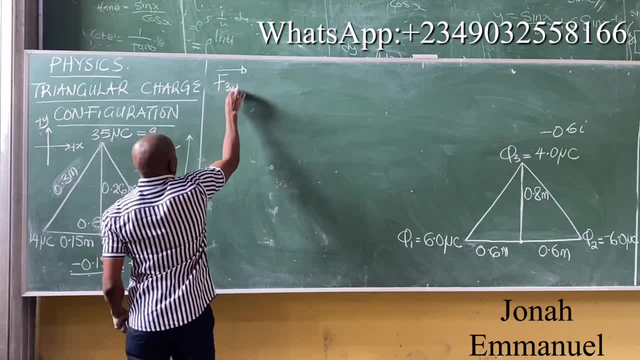 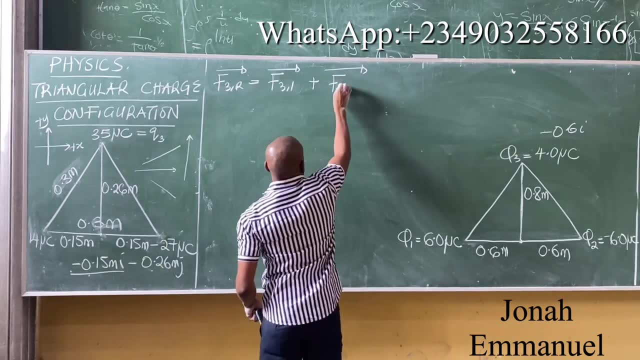 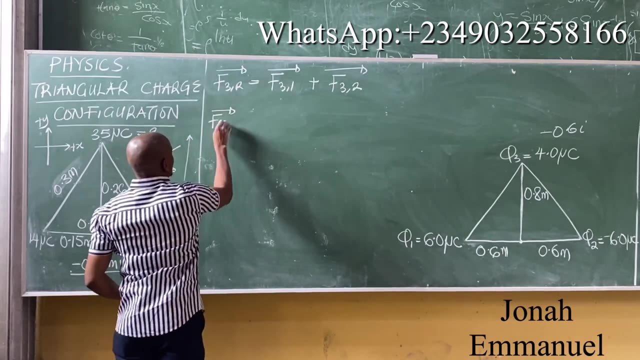 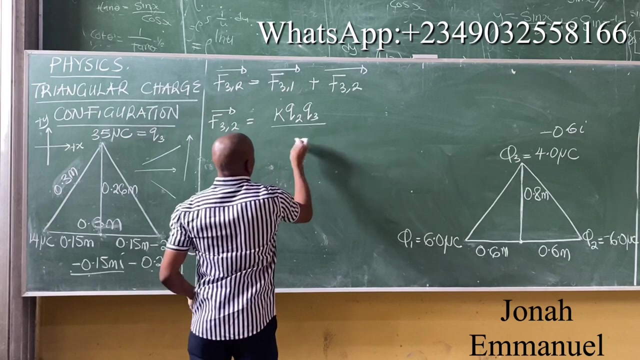 that becomes f of f3, resultant, which is equal to what there, f31 plus f32. um, let me pick f32, so you go on this one. yeah, let me pick up f32. we know that f32 from columns. that becomes what there k, q2, q3, all the water. 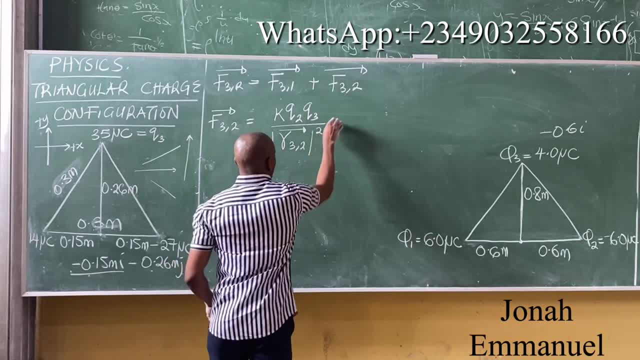 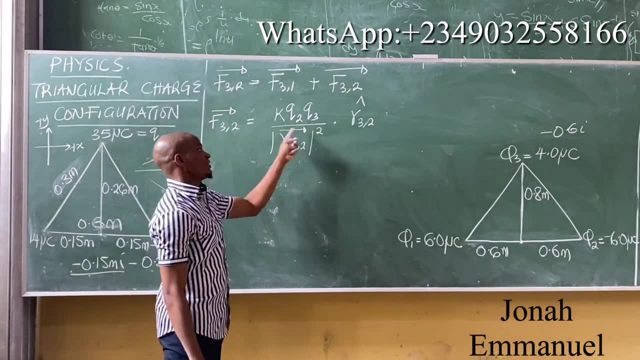 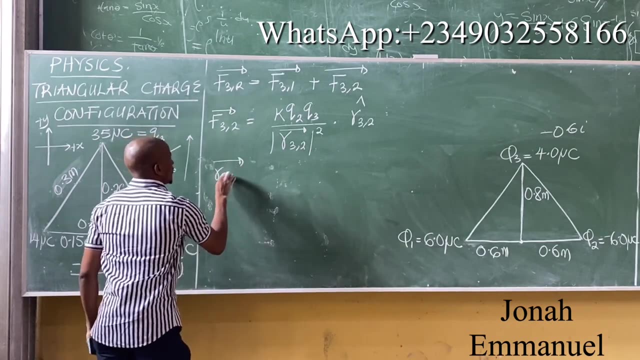 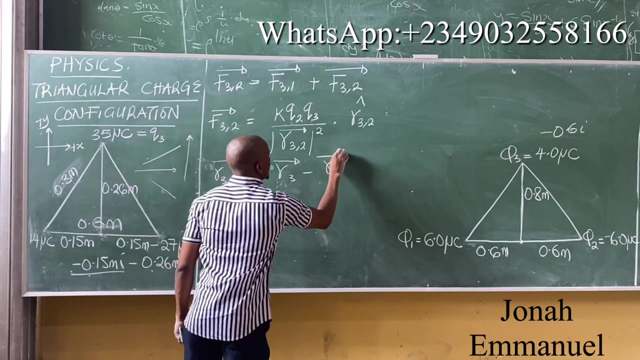 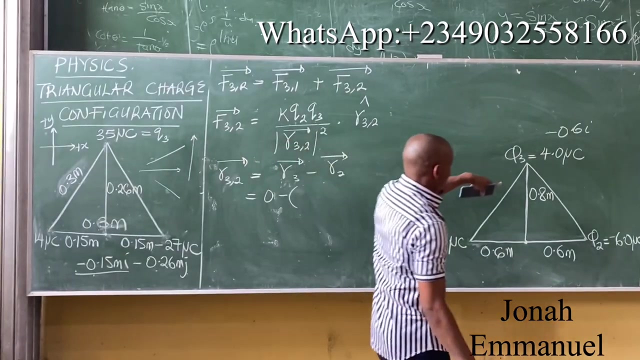 three, two, all water, dot, dot what? i explained this stuff in the last class. why does he think q3, q2, no problem, it's the same thing. let's look at r32. what is r32? what's r32? r32 becomes r3 minus r2. r3 is zero minus what's r2. look at this: this is r3. 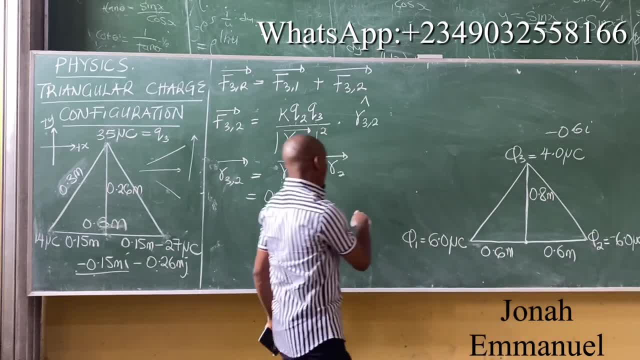 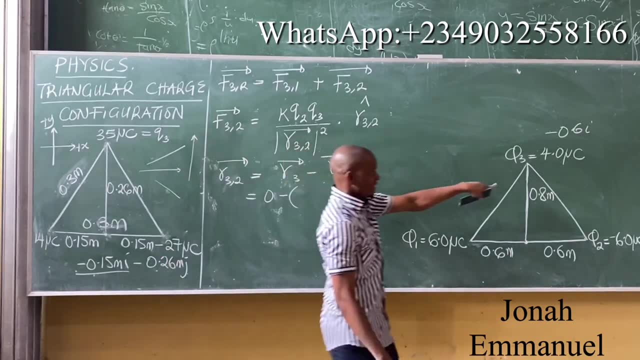 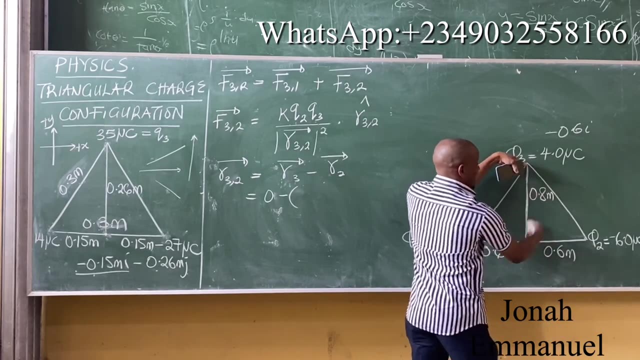 so when they say r2 is minus, now for this is here, replace r3 for r2. so here becomes my datium. so, having zero minus, i'm at this point r3, move to r2. for me to move to r2, observe that i've been given this distance here as 0.8, so no need for. 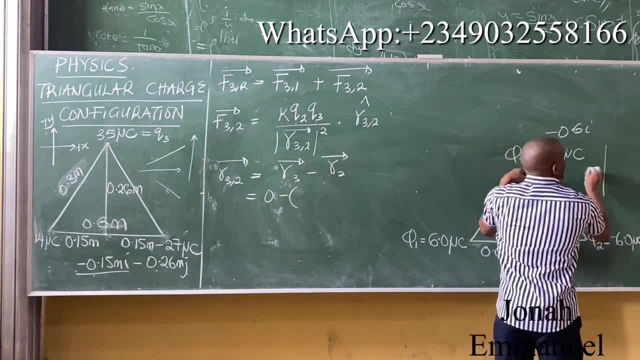 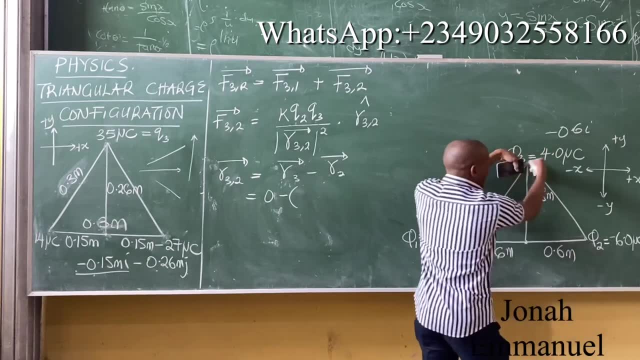 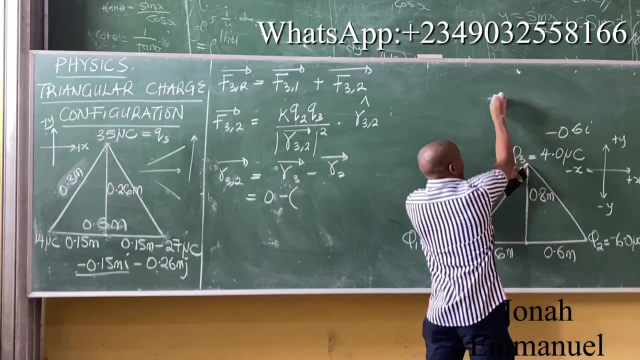 Pythagoras theorem again from here, come down this way. check your cartesian corvette again: plus x, plus y, minus y, minus x. I have to move downwards. If I'm moving downwards, that becomes negative of j, So it becomes minus. this one here: 0.8 meters j. 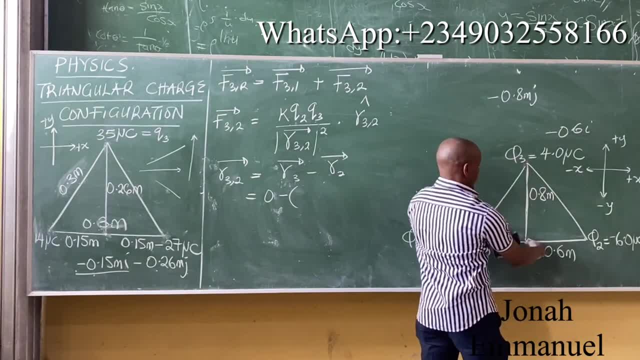 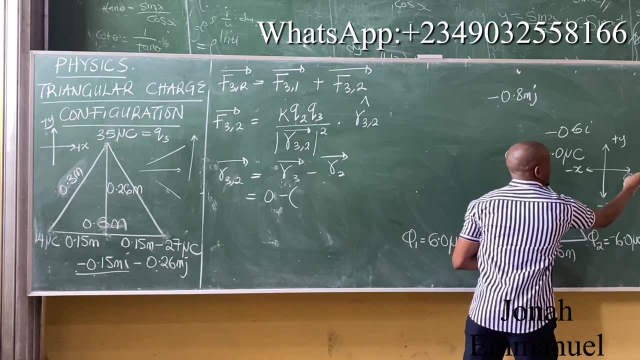 That gives me from here to here. I'm now at this point. From here, if I'm going to Q2, I have to move to the right. Moving to the right becomes what there Positive, So it becomes plus this value here. 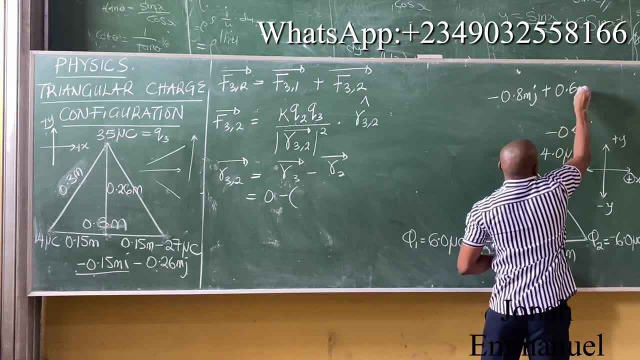 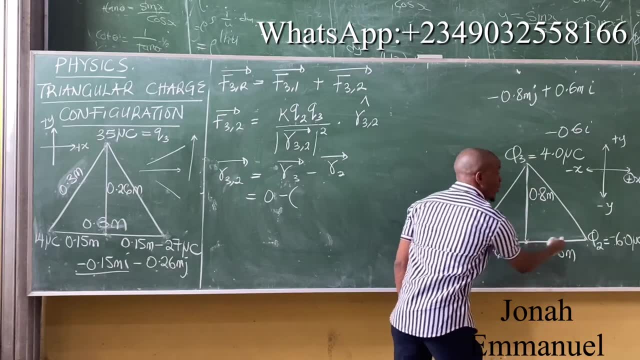 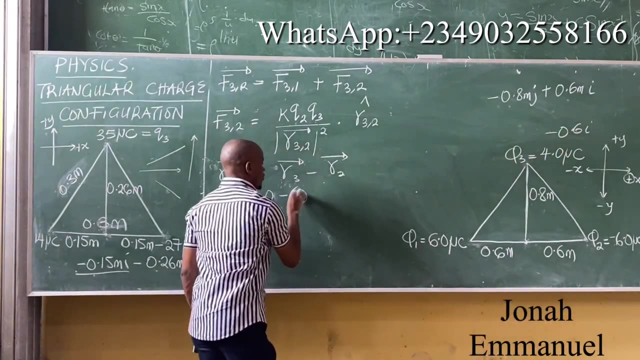 0.6 meters. what there R- Although I have to pass through j first before r When it comes to arrangement place what there I before j. So it becomes what there? 0.6 meters. i Next up, minus 0.8 meters j.